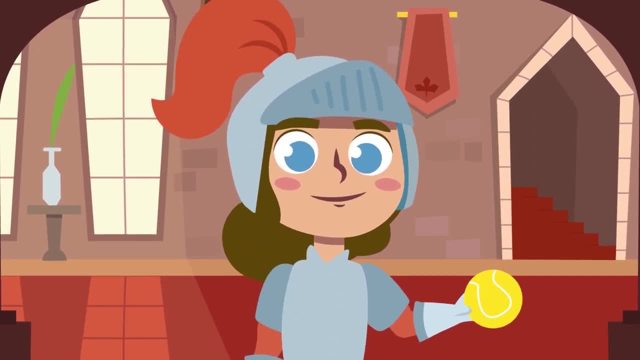 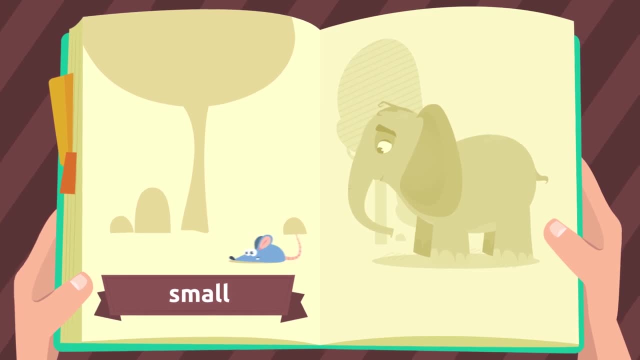 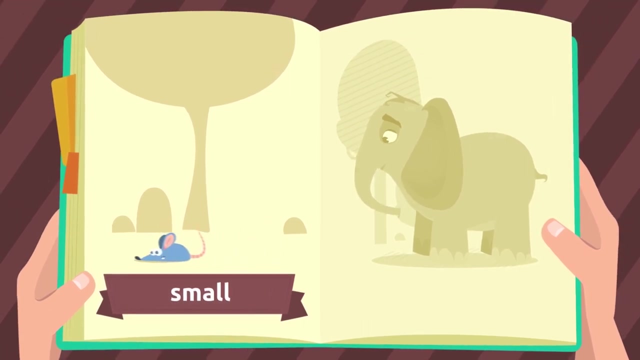 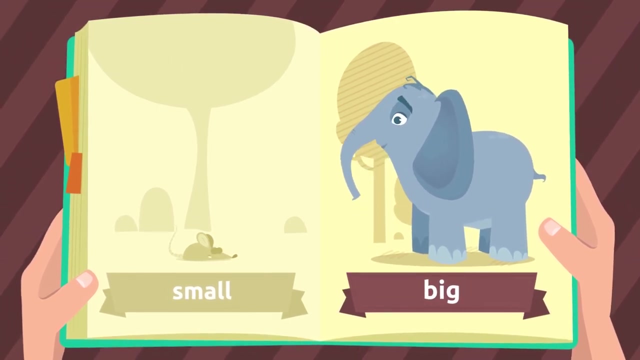 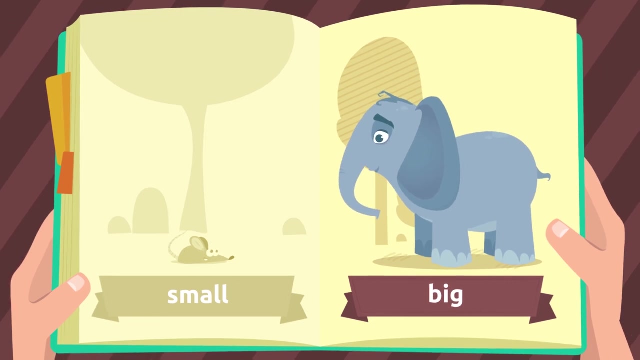 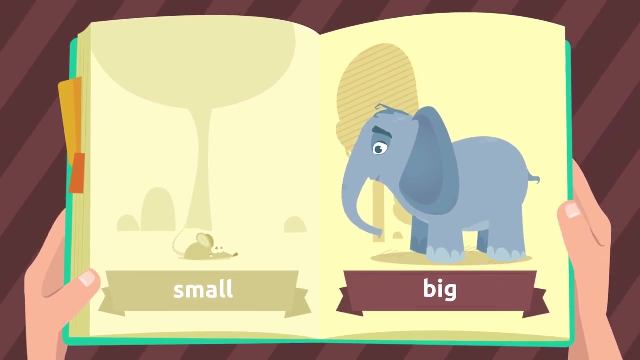 different animals. Come on, let's begin. This mouse is small, Small, Repeat after me, Small, But this elephant is big, Big, Repeat after me: Big, Small, Big, Small, Big. This turtle is slow, Slow. 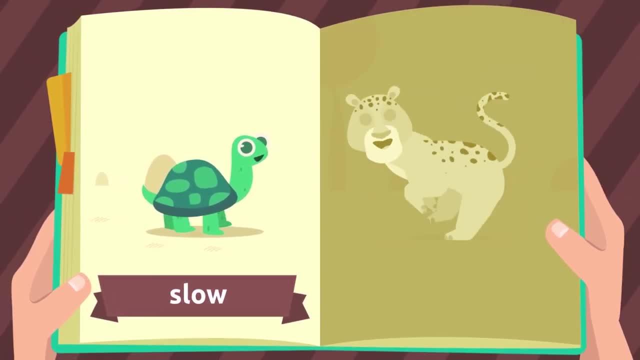 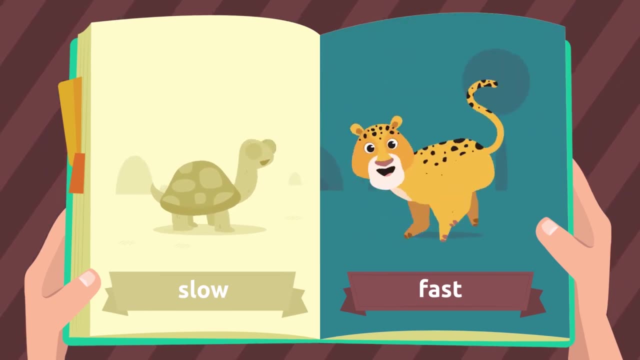 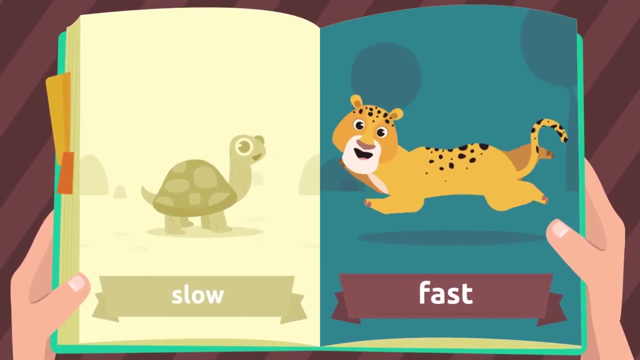 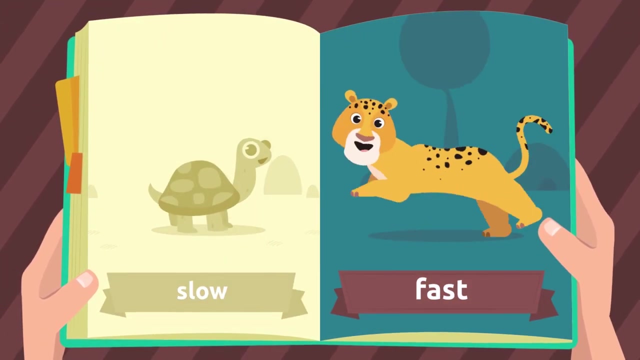 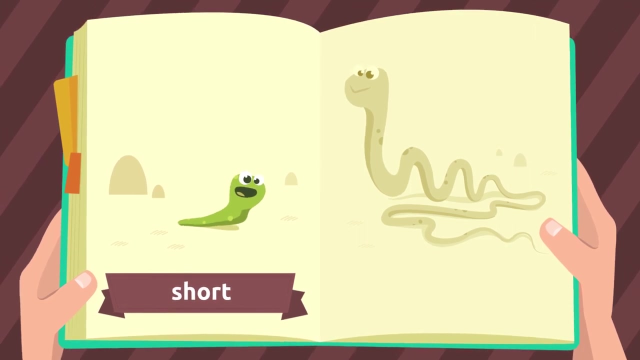 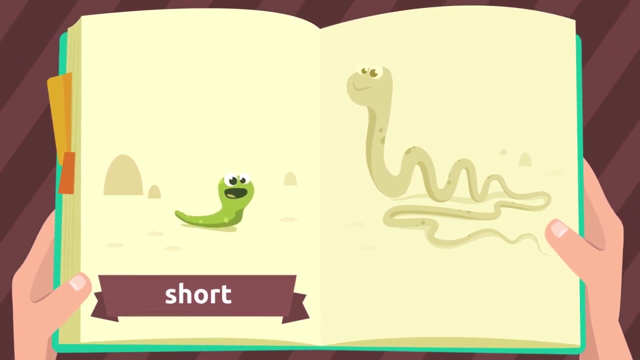 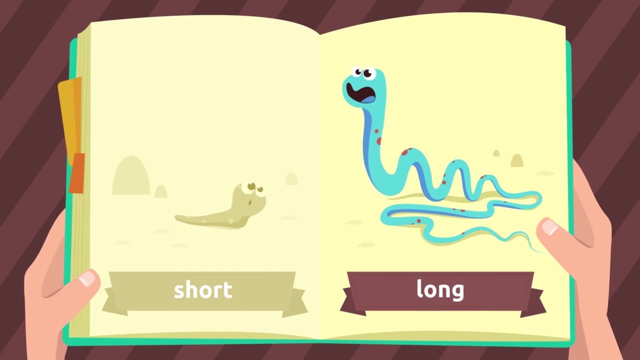 Repeat after me, Slow. And this leopard is fast, Fast, Repeat after me: Fast, Fast, Slow, Fast. This snake is short, Short, Repeat after me: Short, Short. But this snake is long, Long Repeat after me. 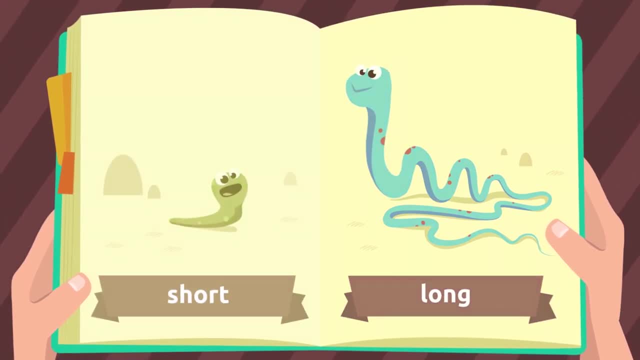 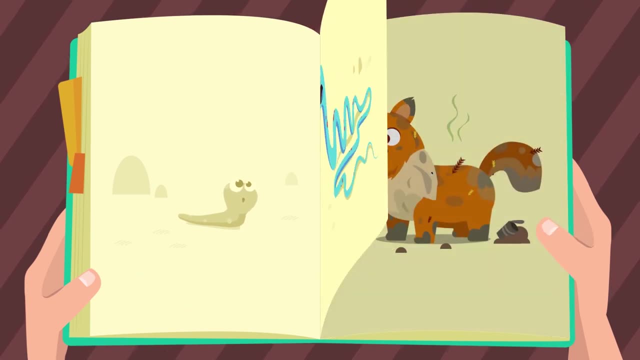 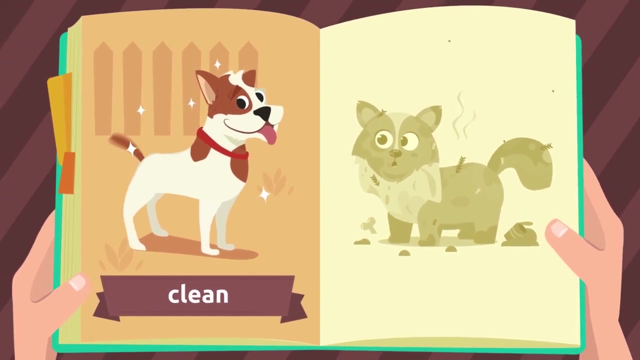 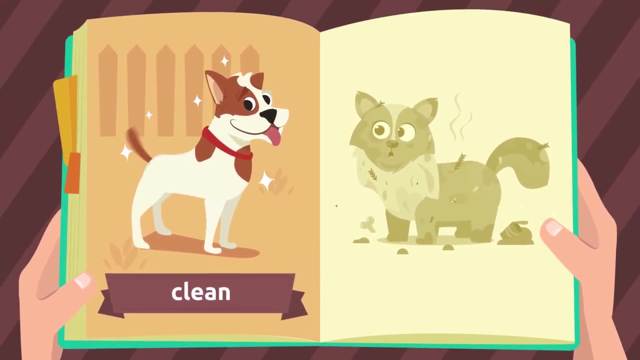 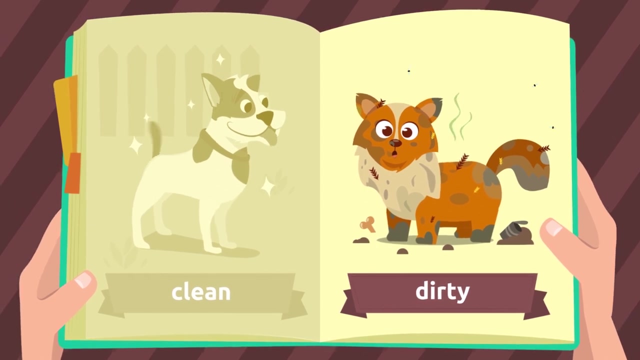 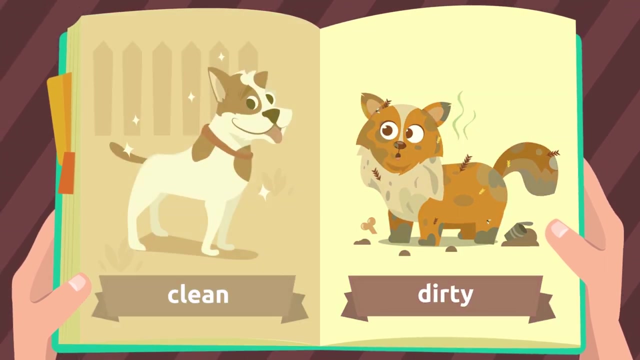 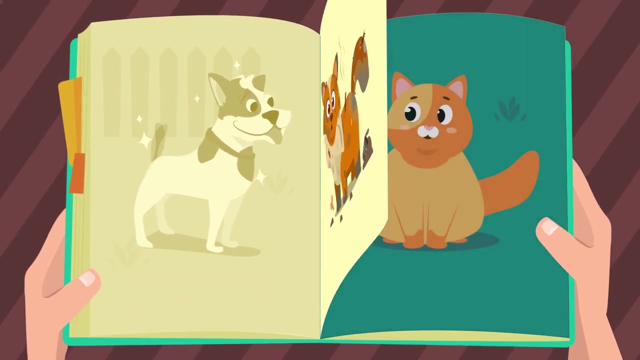 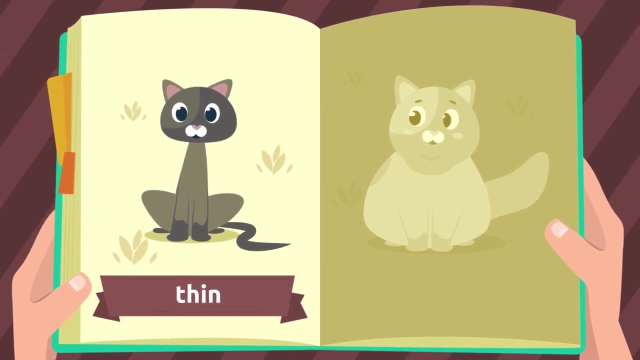 Long, Short, Long. This dog is clean, Clean, Clean, Repeat after me Clean. And this dog is dirty, Dirty, Dirty, Repeat after me Dirty, Clean, Dirty. This cat is thin, Thin Repeat after me. 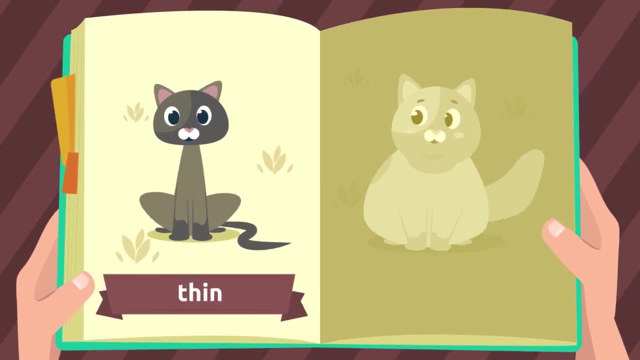 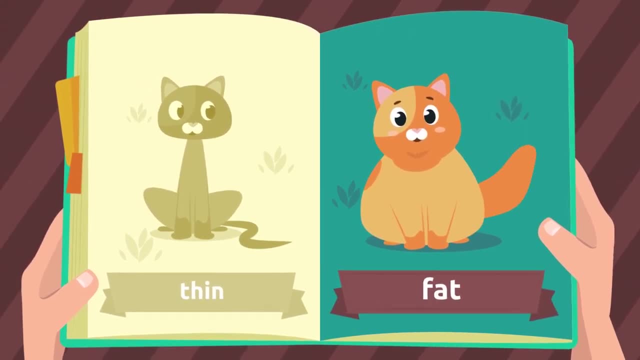 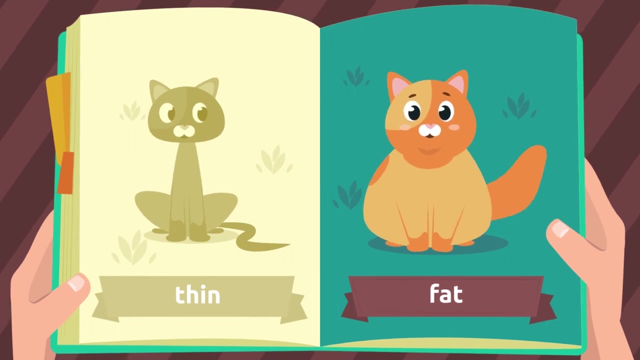 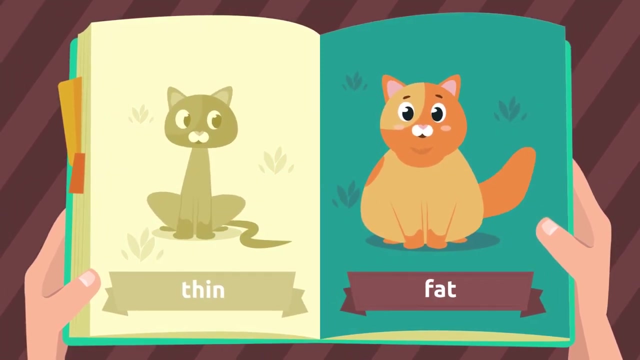 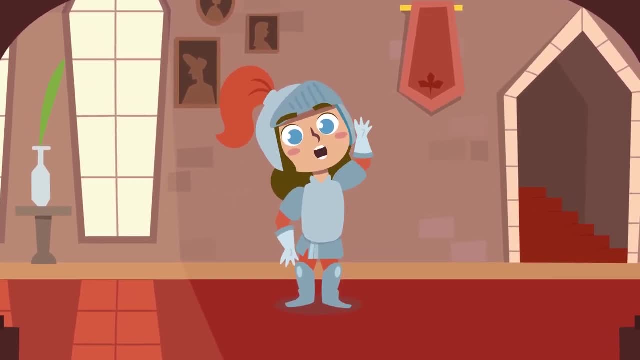 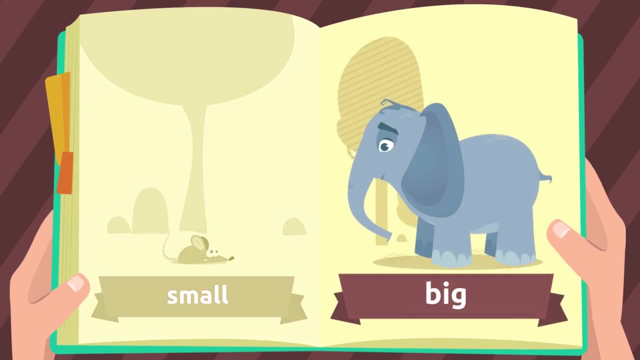 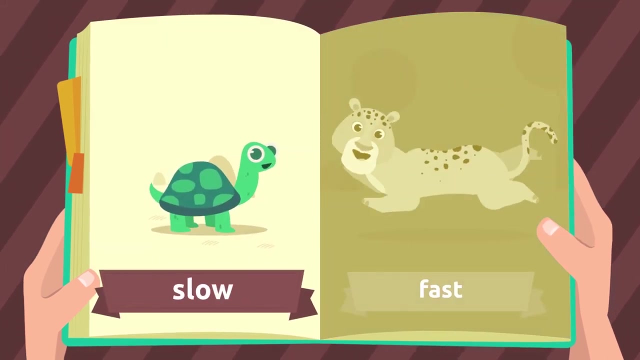 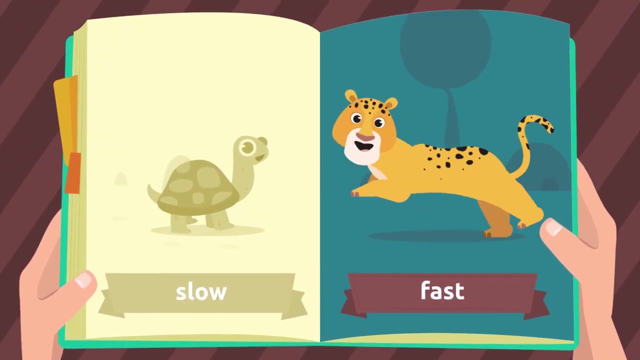 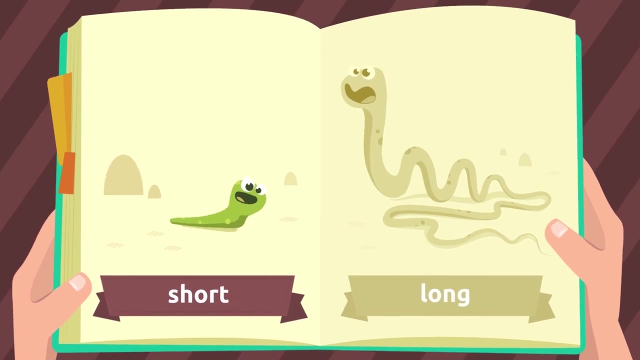 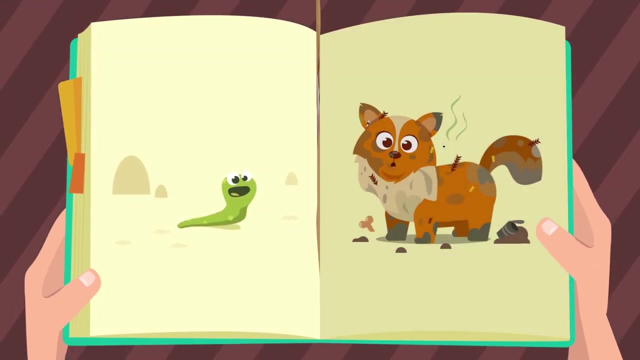 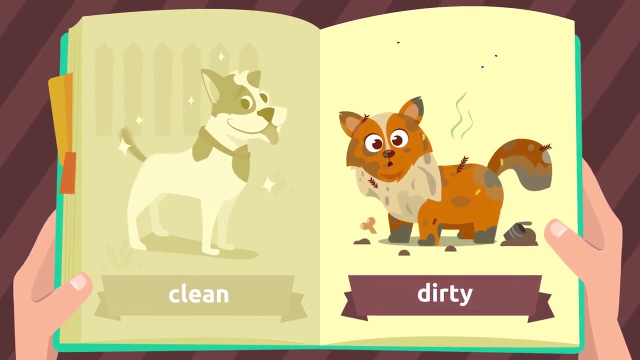 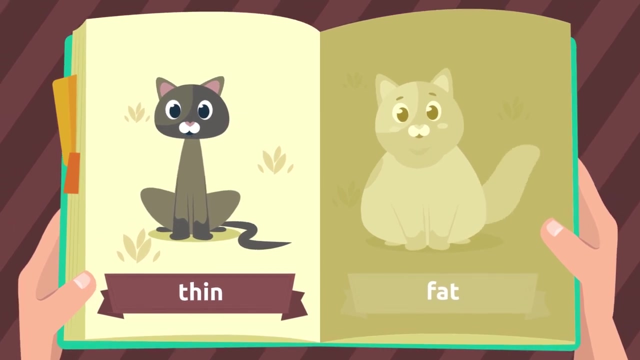 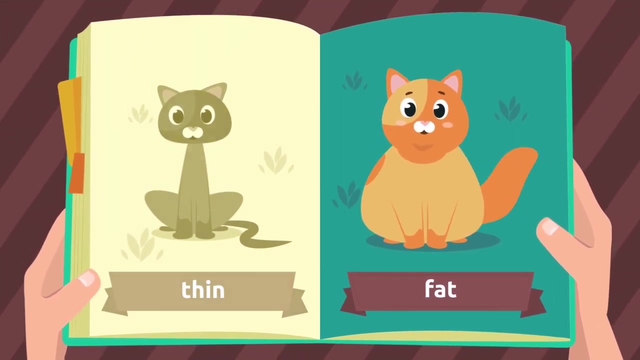 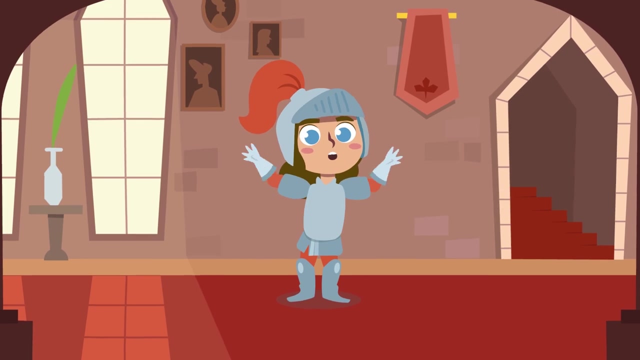 Thin, Thin, Thin, Thin, Thin, Small, Big, Slow, Fast, Short, Long, Clean, Dirty, Thin, Fat, Fat, Awesome. Adjectives are super fun. In this video, we've learned a lot about them with some animals. 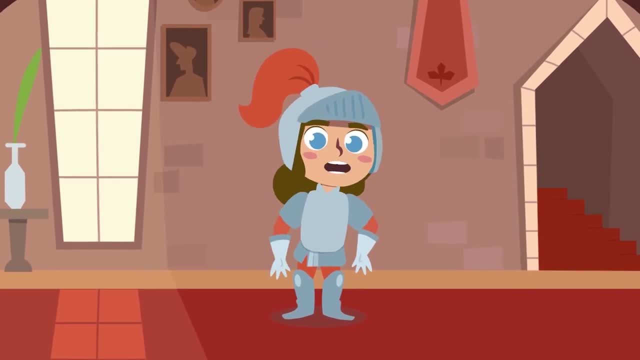 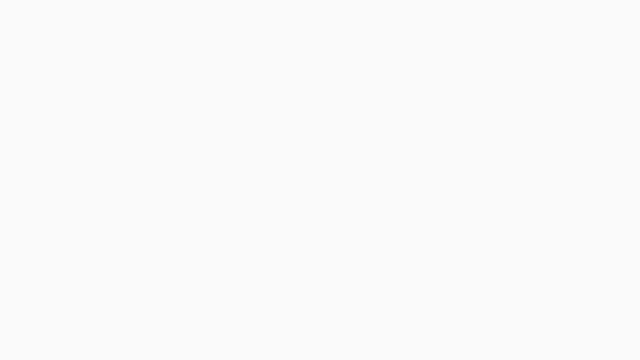 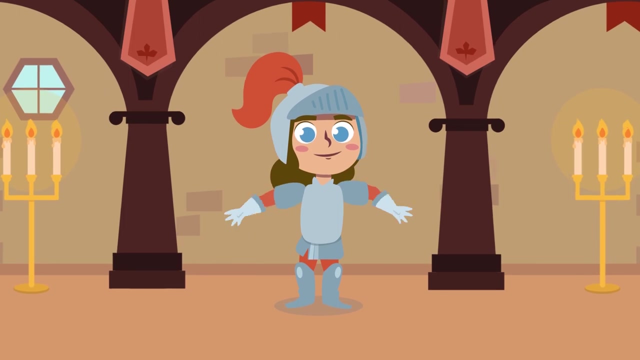 In the next one we'll learn some more, but this time with people. Don't miss it. How are my word lover friends? Today we'll continue learning more adjectives. What do you say? Do you remember what they are? 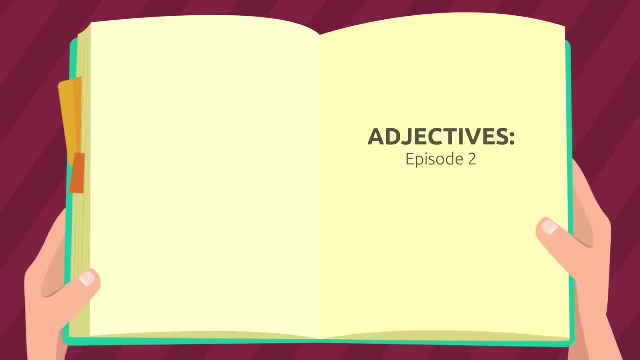 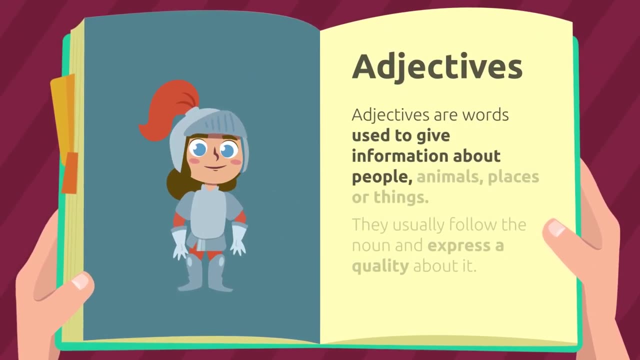 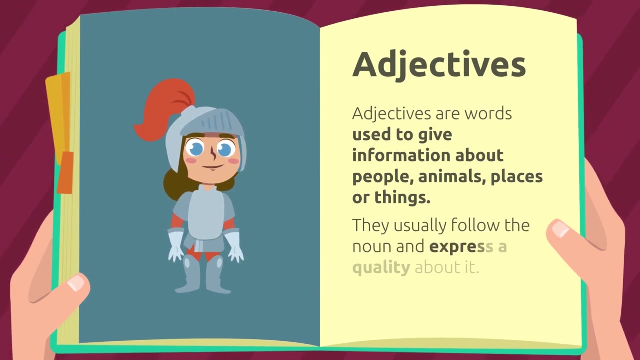 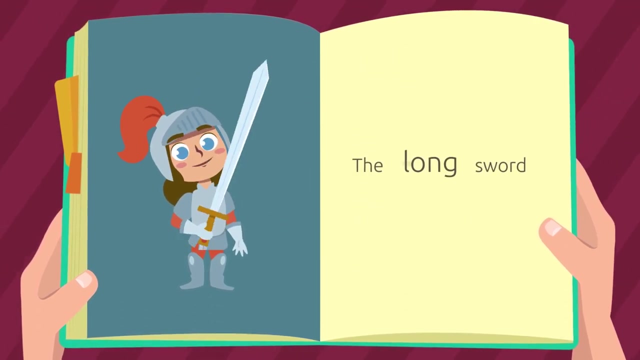 If not, I'll remind you. Adjectives are words used to give information about people, animals, places or things. They usually follow the noun and express a quality about it, For example, in the sentence the long sword. long would be the adjective, because it tells us what the sword is like. 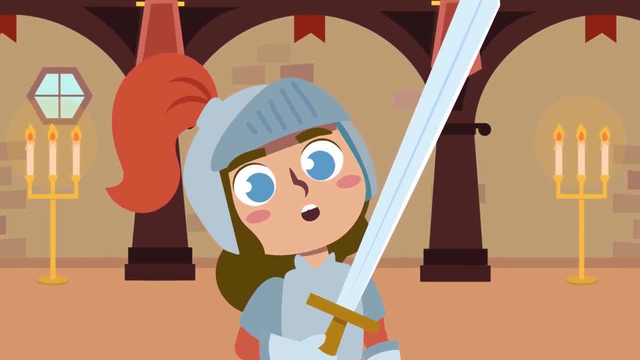 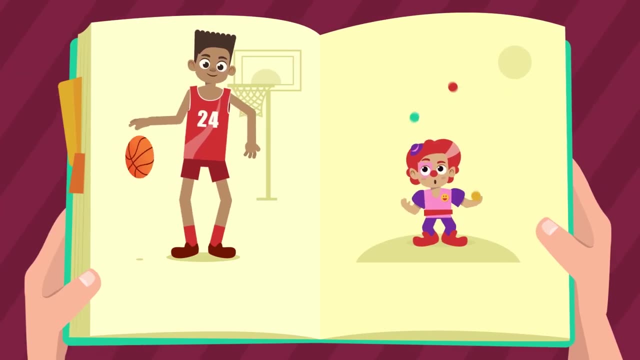 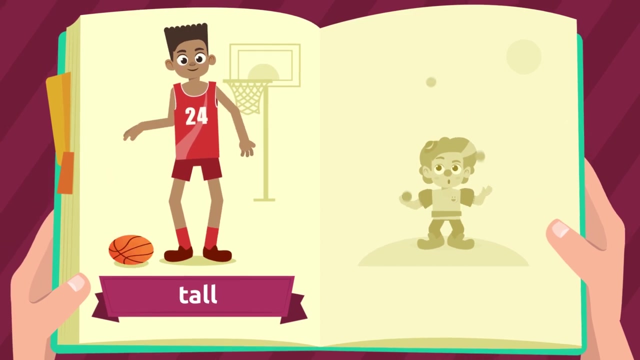 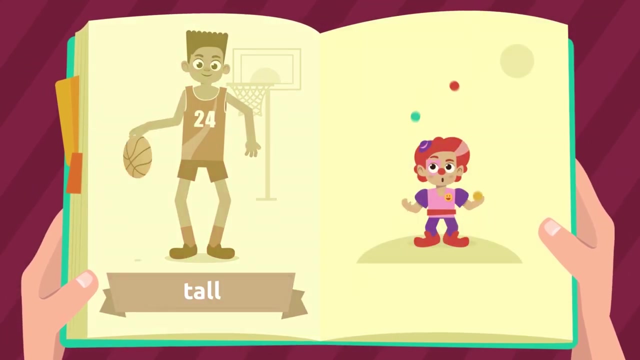 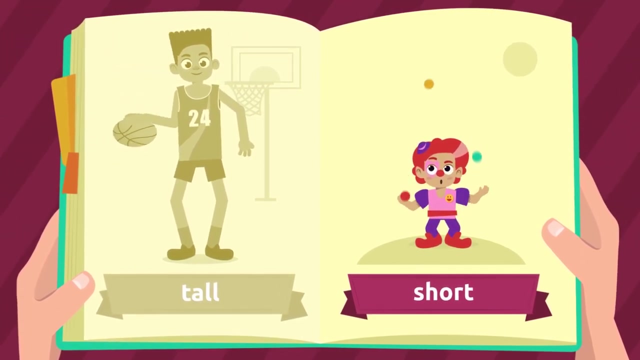 In this video, we're going to learn about some adjectives that describe qualities about different people. Here we go. This basketball player is tall- Tall, Repeat after me, Tall. But this clown is short- Short, Repeat after me. 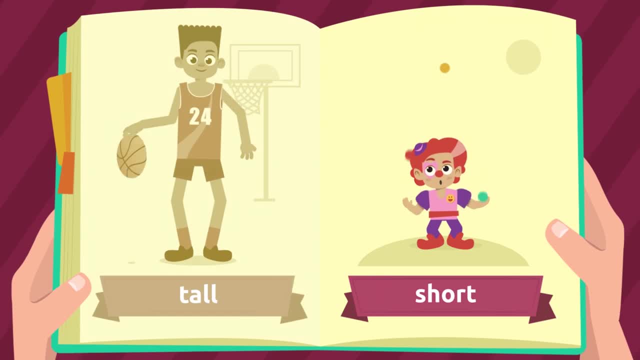 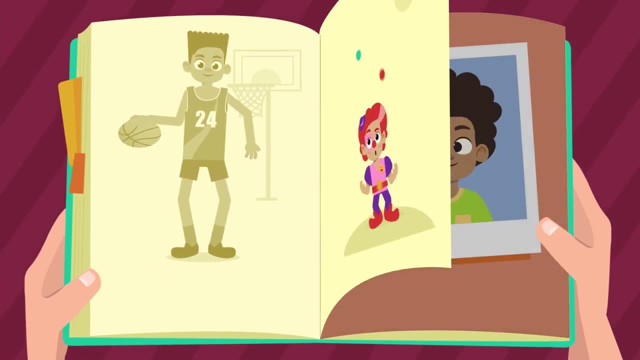 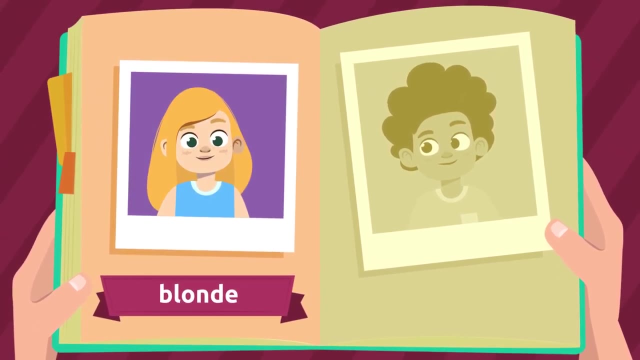 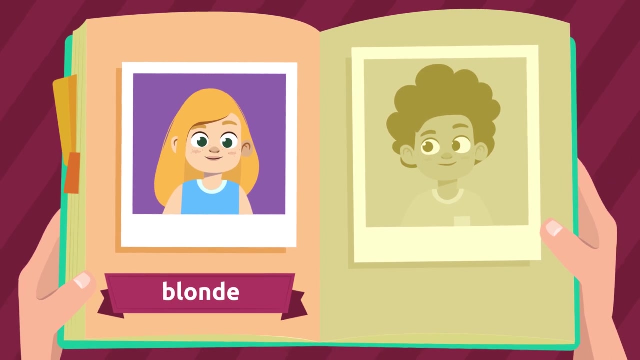 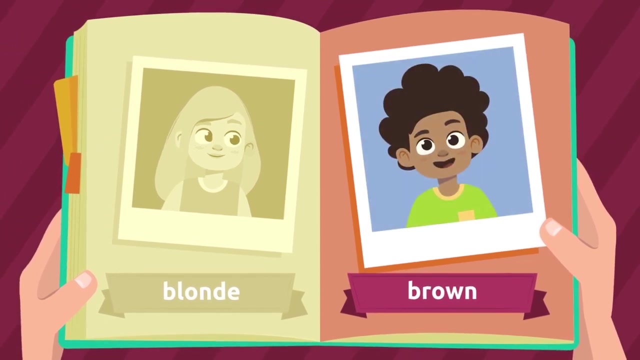 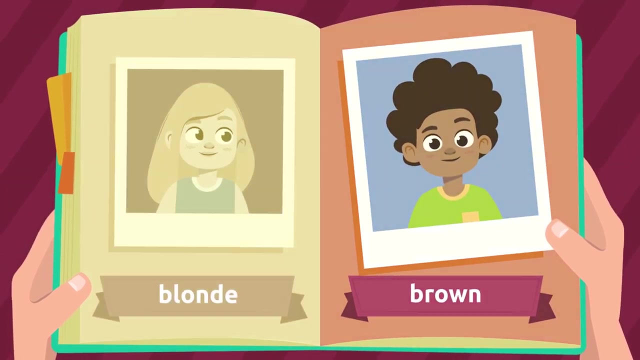 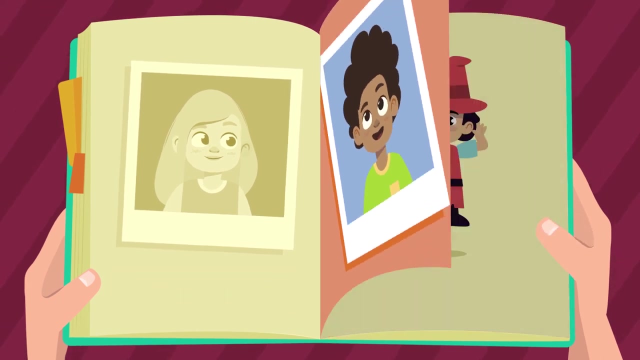 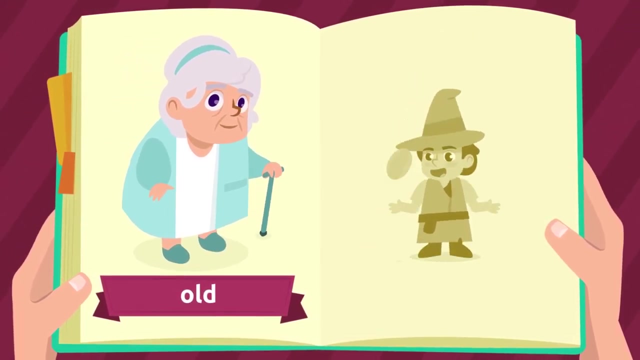 Short, Tall Short. Paula has blonde hair- Blonde- Repeat after me, Blonde, Blonde. And Miguel has brown hair- Brown- Repeat after me: Brown, Blonde, Brown. This grandmother is old, Old- Repeat after me Old. 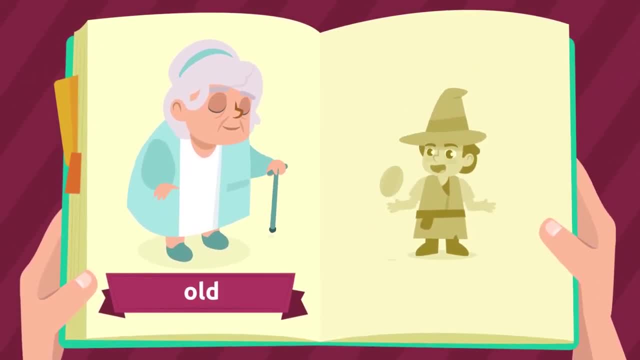 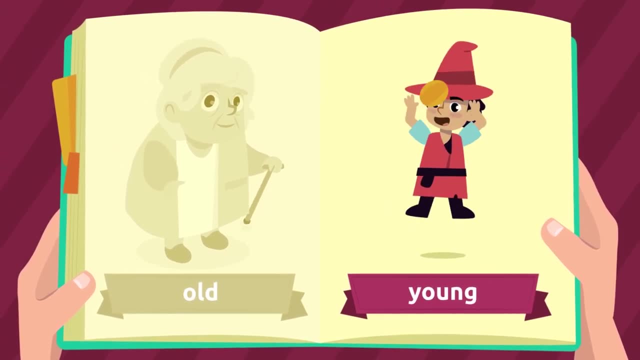 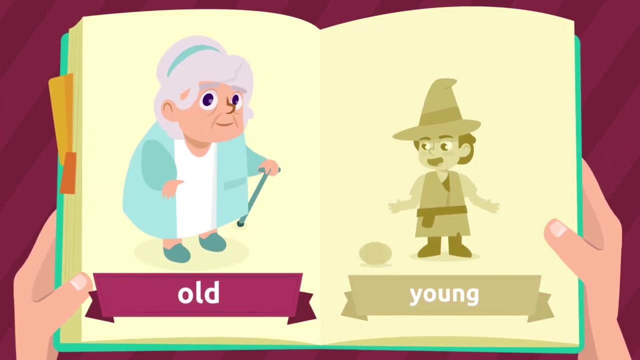 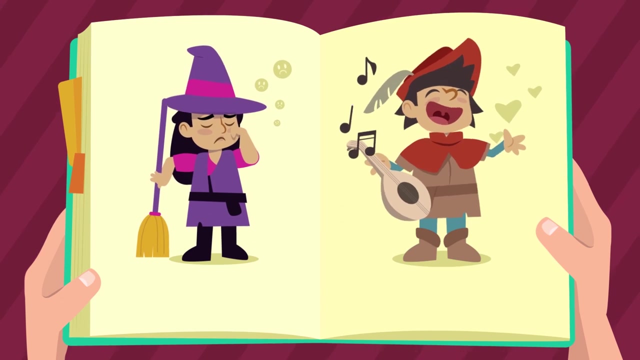 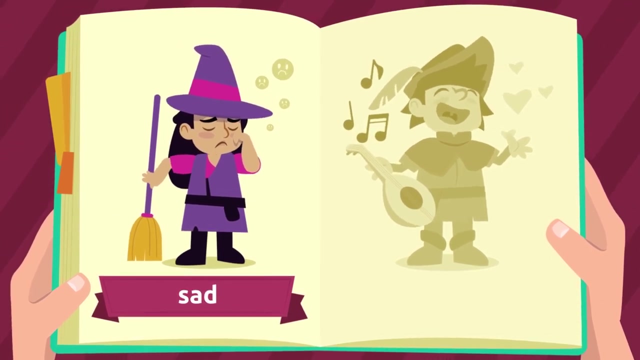 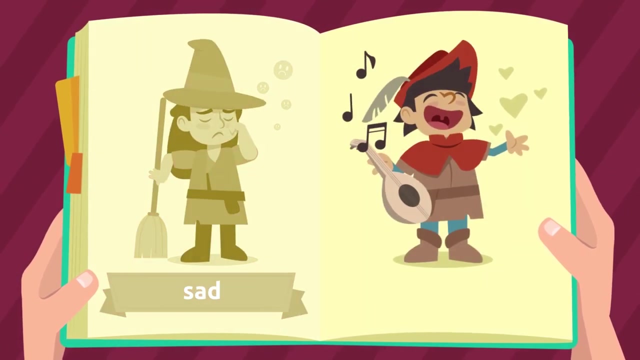 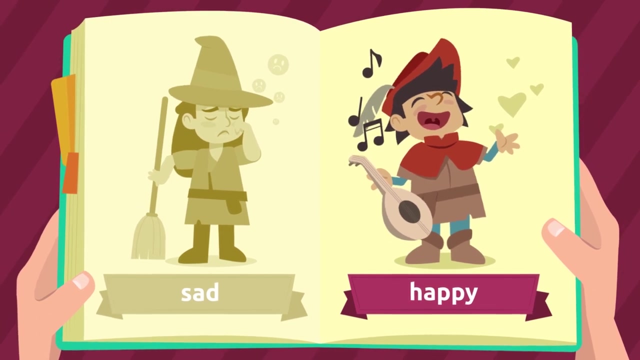 Old, Old, Old. And this boy is young, Young- Repeat after me- Young, Old, Young. This witch is sad, Sad, Repeat after me, Sad, Sad, Sad. But this musician is happy, Happy, Happy. 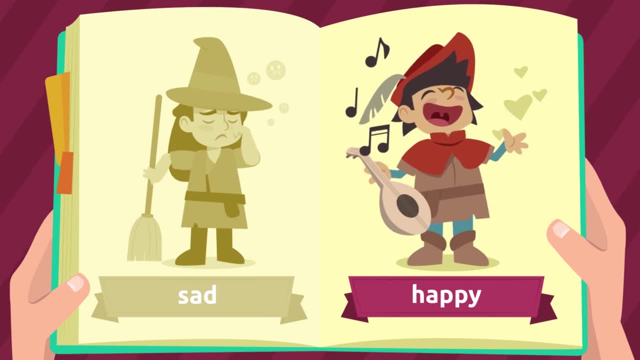 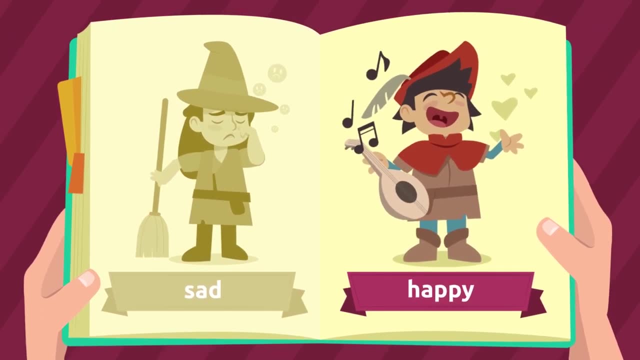 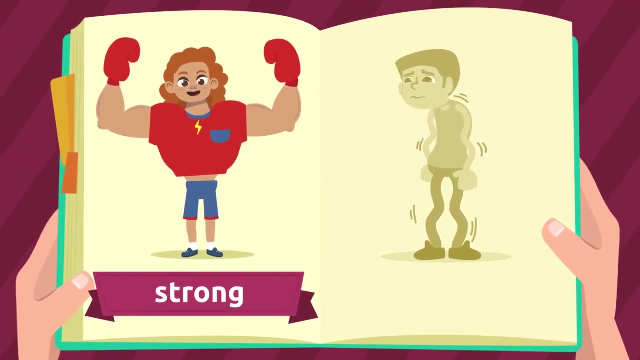 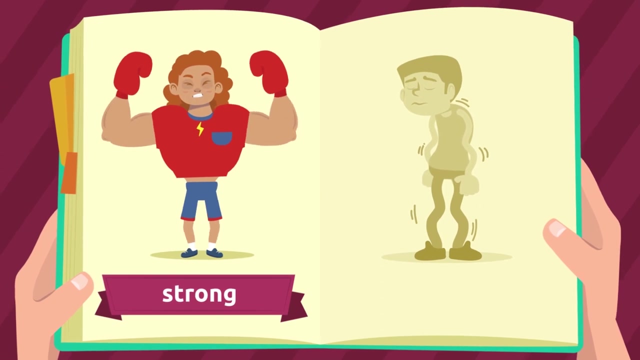 Repeat after me: Happy, Sad, Happy, Happy. This boxer is strong, Strong, Happy, Luv, Got it Great. Happy, Strong, Happy, Normal. Repeat after me: Strong, Good Puppy. But this boy is weak. 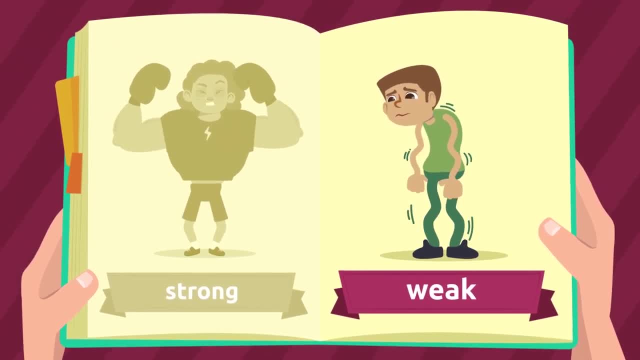 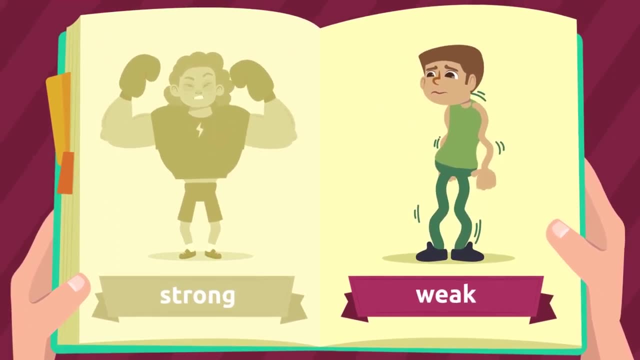 Buffy, Weak, Weak, Sometimes sitting in love. Do you love yourself? It's too much. Preliminary power: 80.. Up 20.. Ch captain, wydd Up, Up, Up, Up, Up Up. 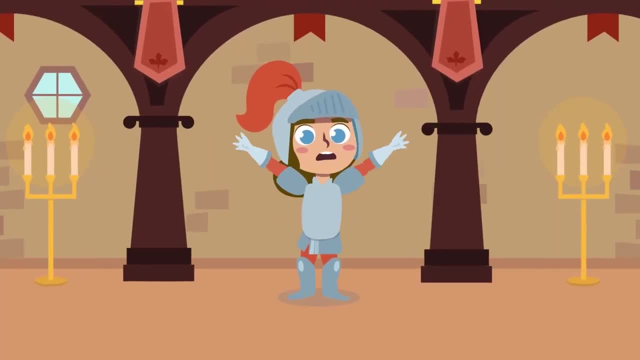 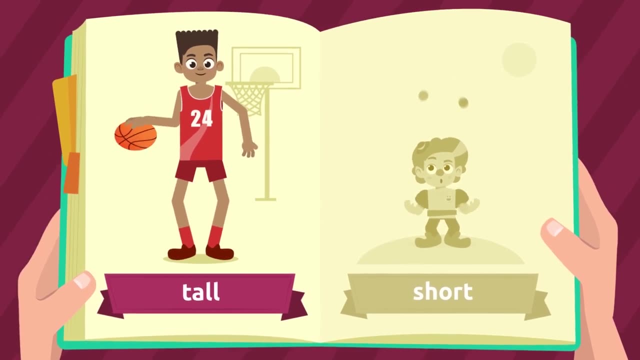 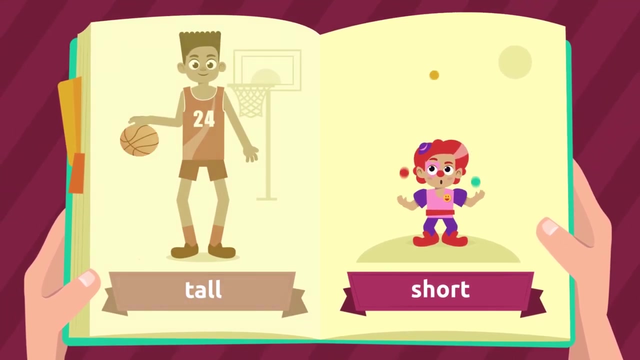 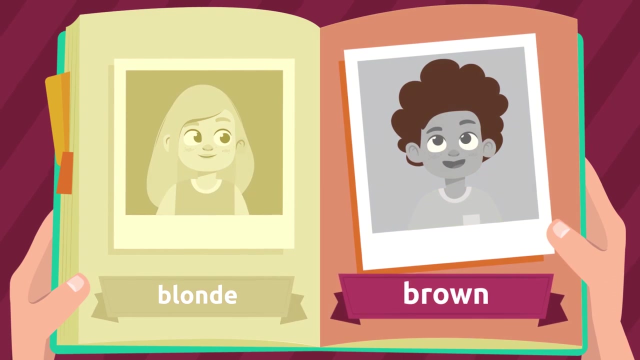 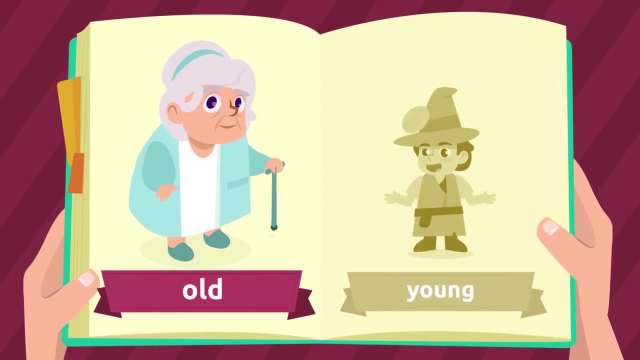 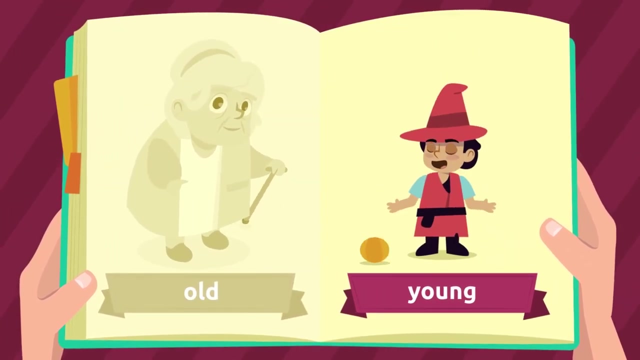 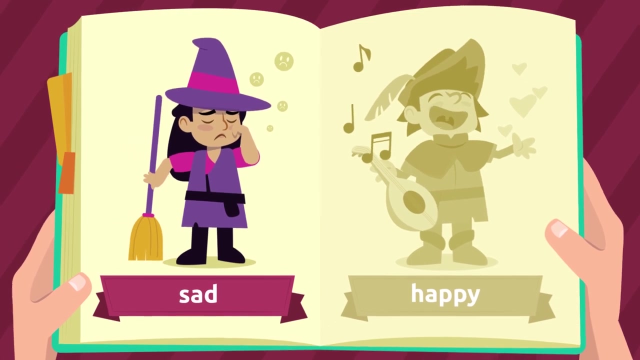 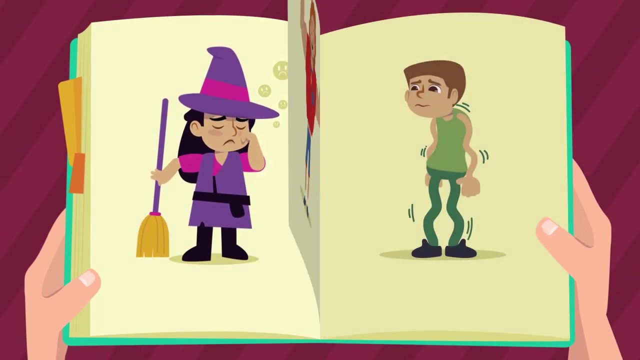 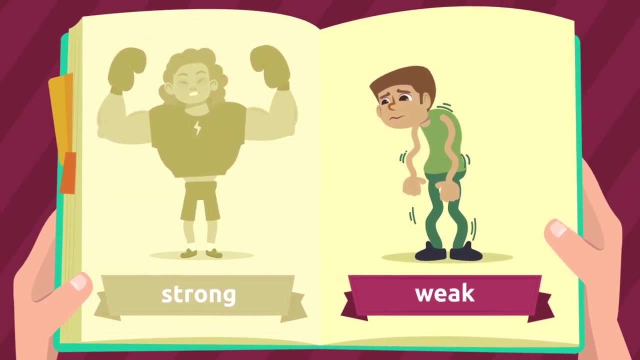 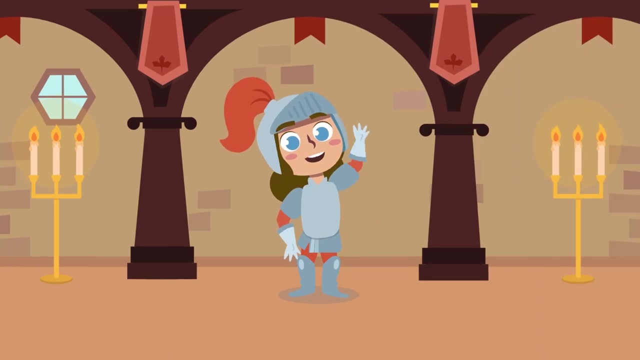 Swab Up, Swprise, Swab. We've learned a lot of adjectives about these friendly people. Let's review them: Tall, Short, Blonde, Brown, Old, Young, Sad, Happy, Strong, Weak, Good job Adjectives are super fun In this video. we've learned a lot about them with some people. 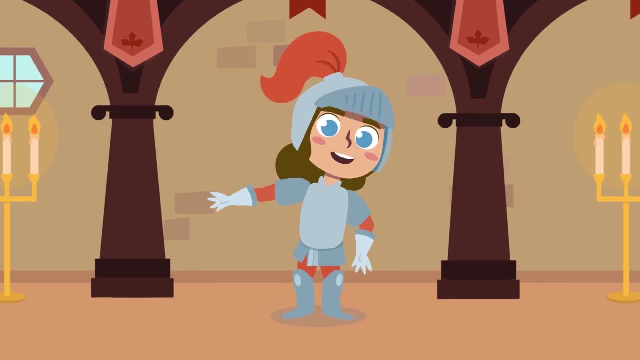 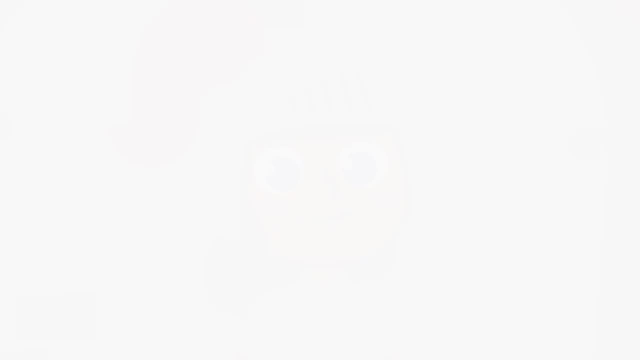 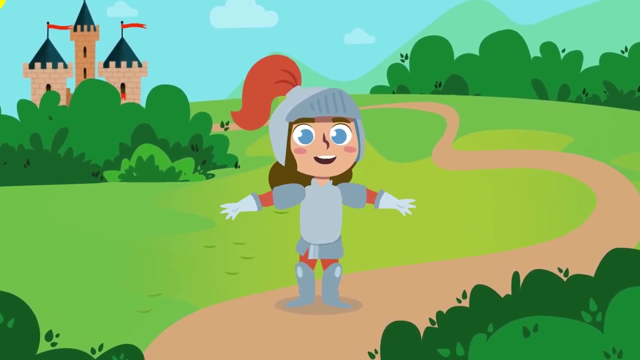 In the next one, we will learn more, but this time with places. Don't miss the next video. How are you my word-lover friends? Today, we will continue learning more adjectives. Today, we will continue learning more adjectives. 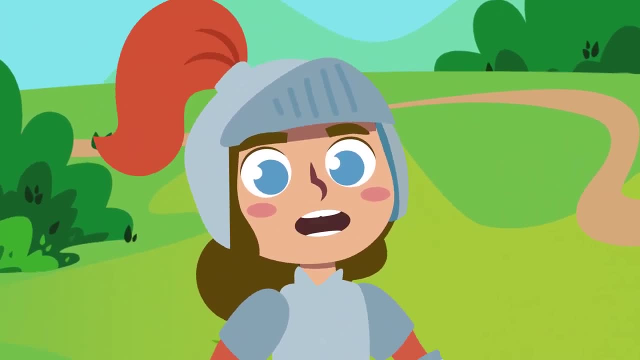 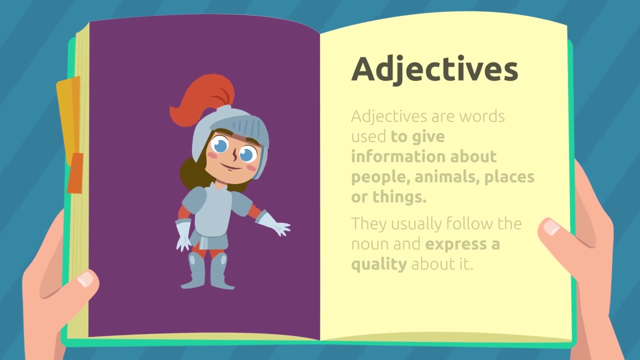 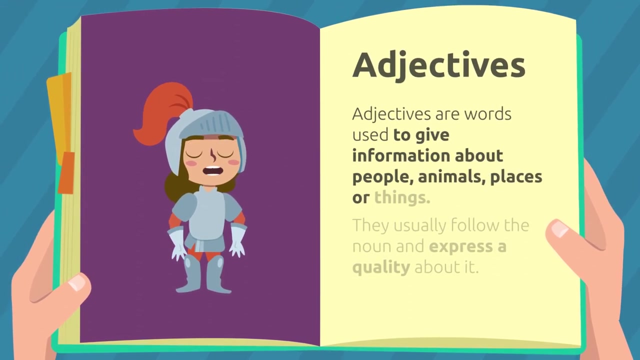 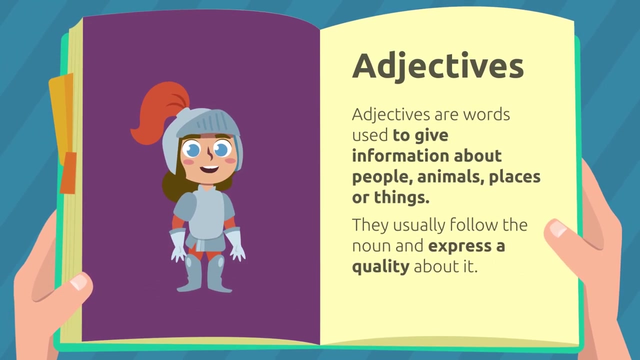 Do you remember what adjectives are? If not, we'll give you a hand. Adjectives are words used to give information about people, animals, places or things. They usually follow the noun and express a quality about it, For example, in the sentence the pretty flower. 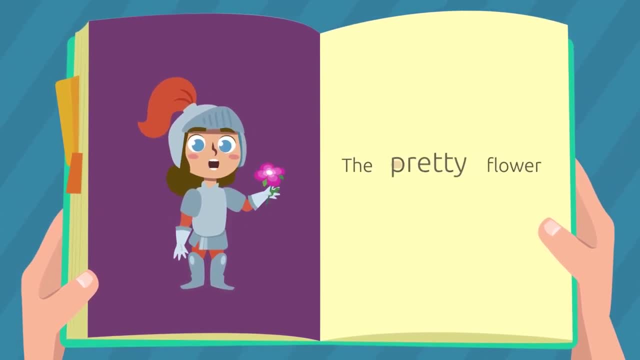 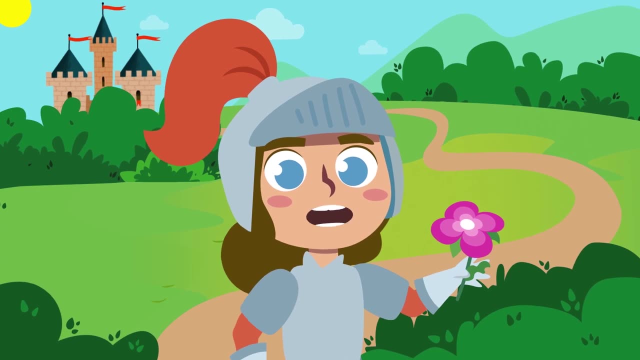 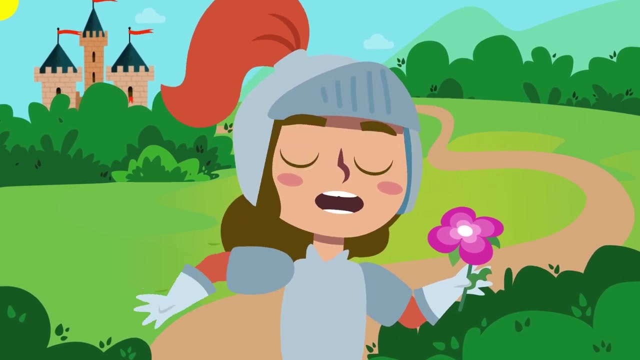 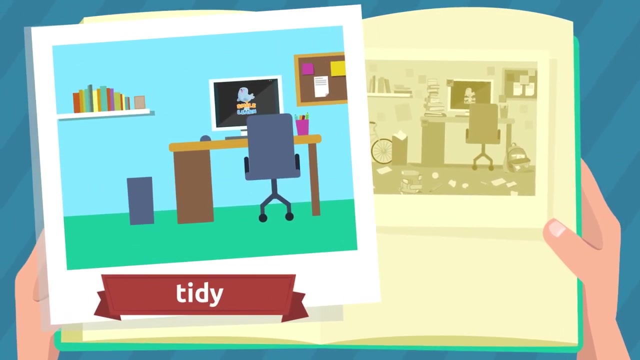 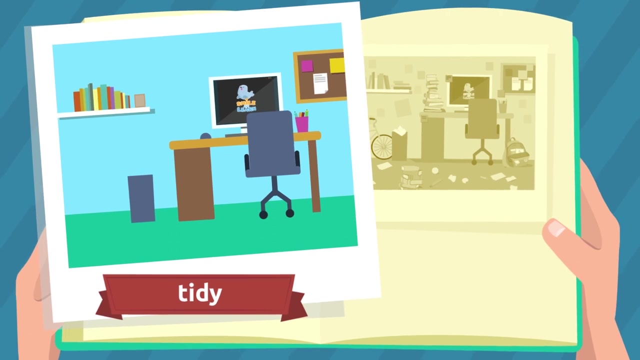 Pretty means pretty, not like would be the adjective, because it tells us what the flower is like. in this video, we're going to learn some adjectives that describe qualities about places. will you stay and learn with me? the room is tidy, tidy- repeat after me: tidy, but 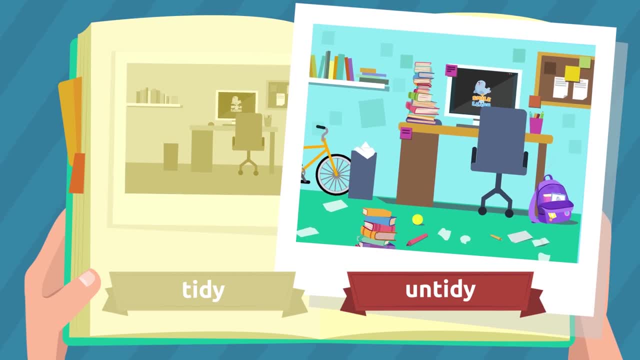 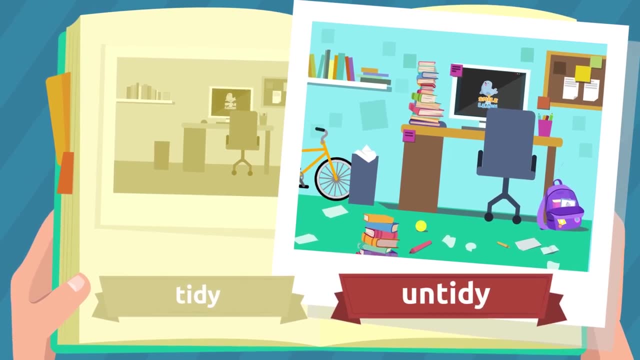 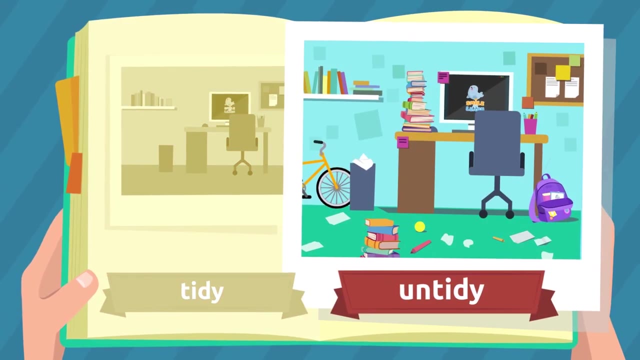 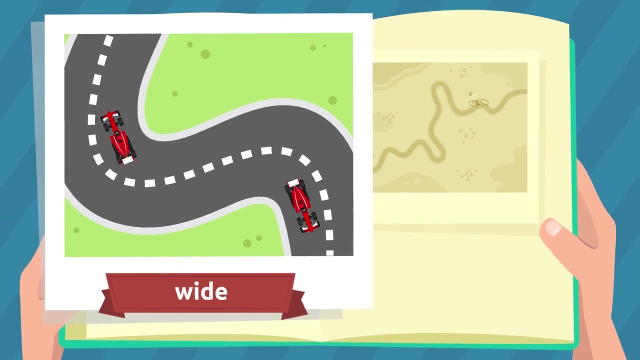 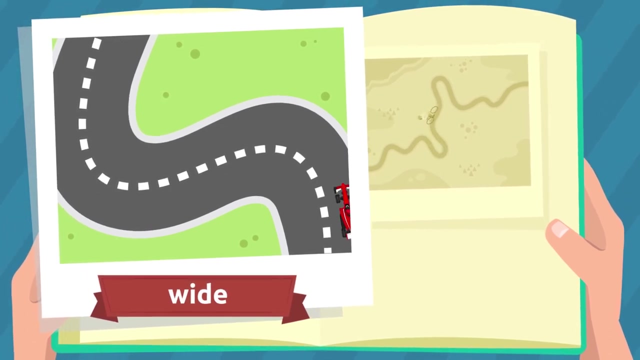 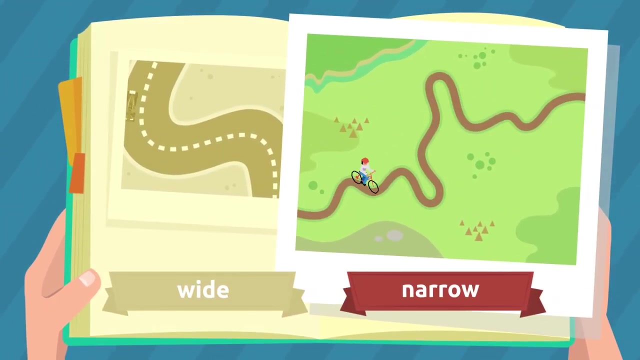 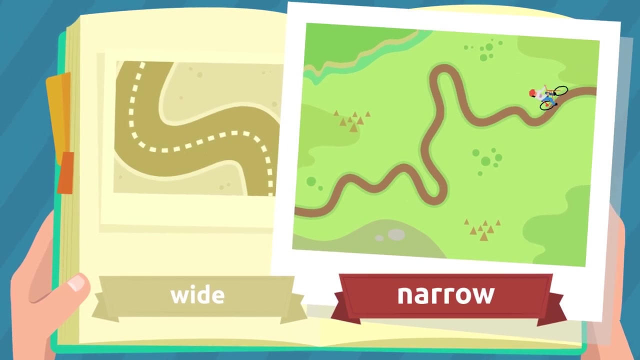 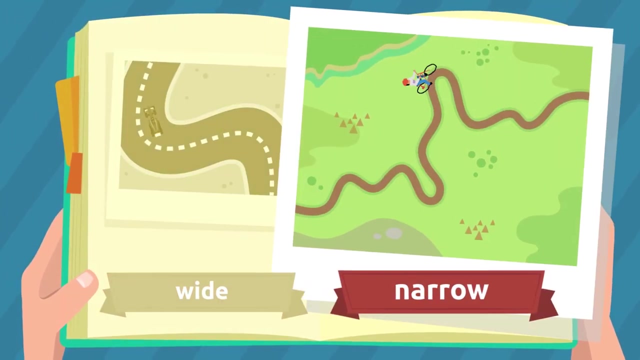 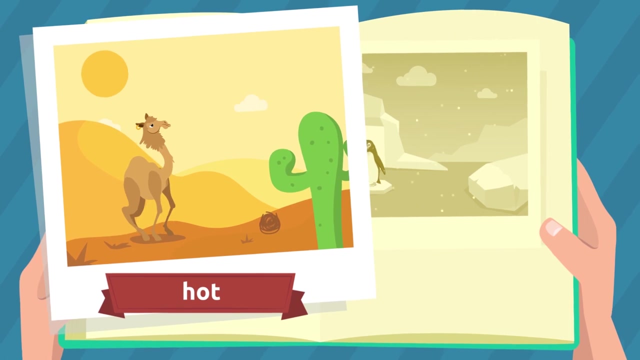 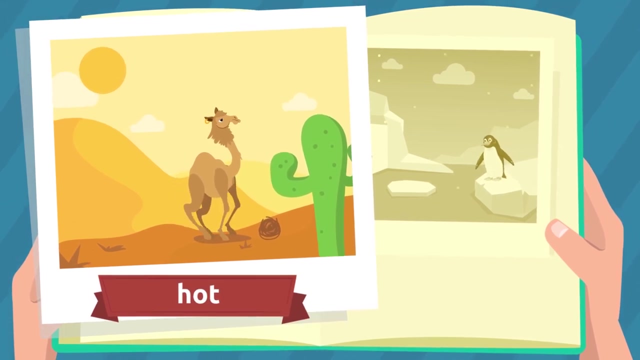 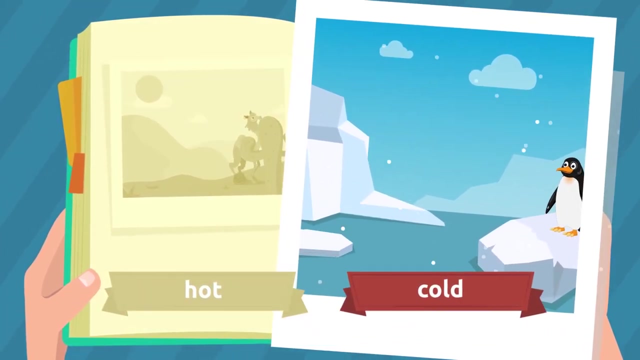 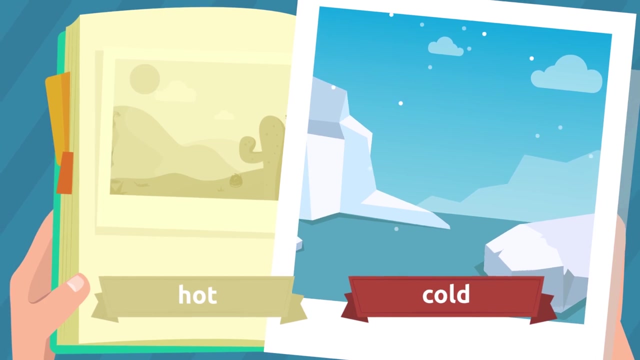 this other room is untidy, untidy, repeat after me untidy, tidy, untidy. this road is wide, wide, repeat after me wide. and this road is narrow, narrow, repeat after me narrow, wide, narrow. the desert is hot, hot, repeat after me hot, but the South Pole is cold, cold, repeat after me cold. 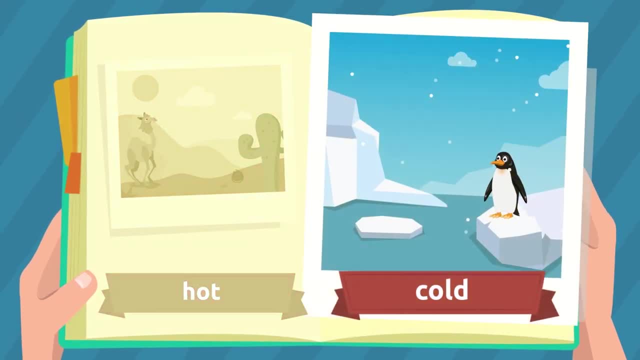 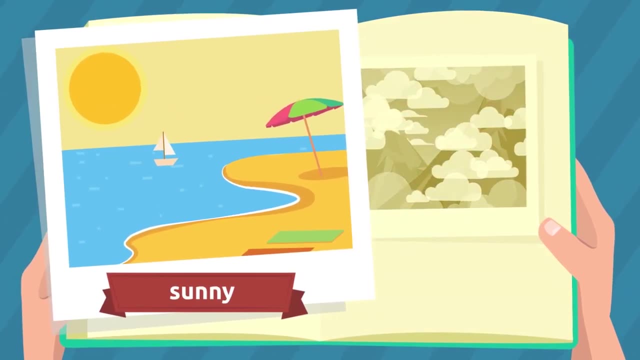 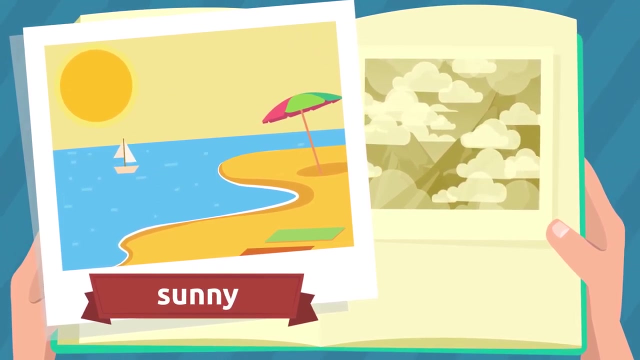 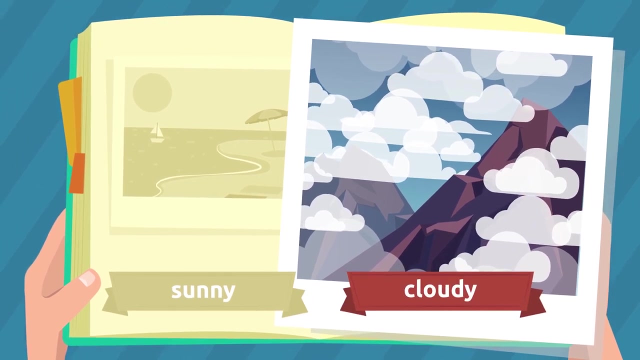 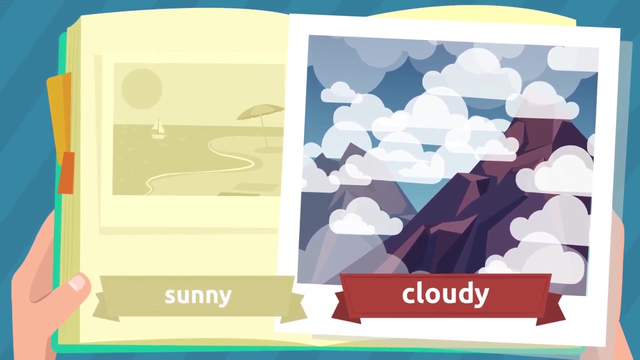 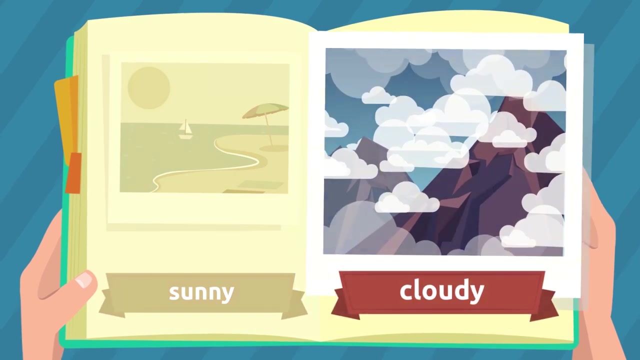 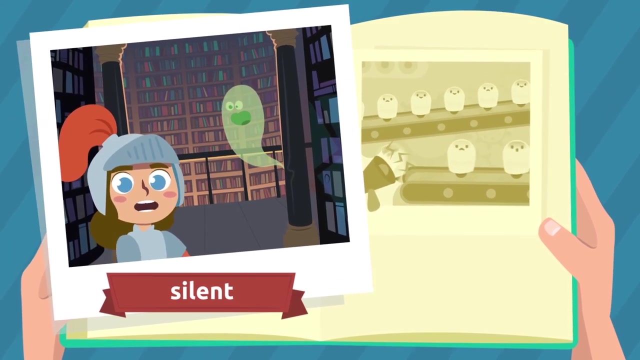 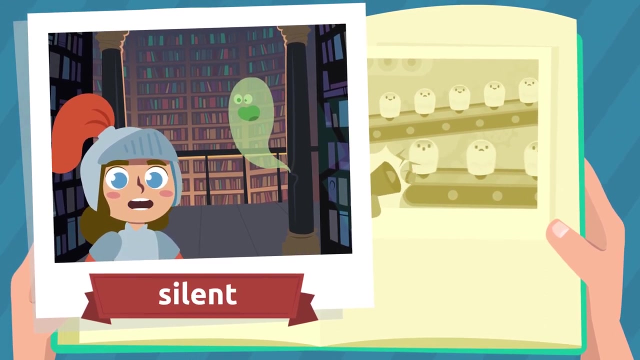 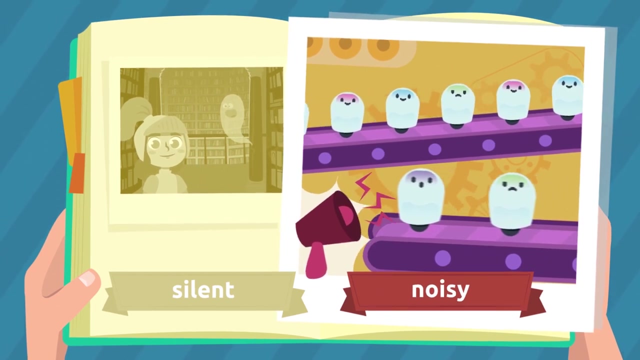 hot, cold. it's a sunny day at the beach- sunny, repeat after me, sunny. and it's a cloudy day in the mountains: cloudy voice, repeat after me: cloudy, Sunny ü. This library is silent, Repeat after me, Silent. But this factory is noisy, Repeat after me. 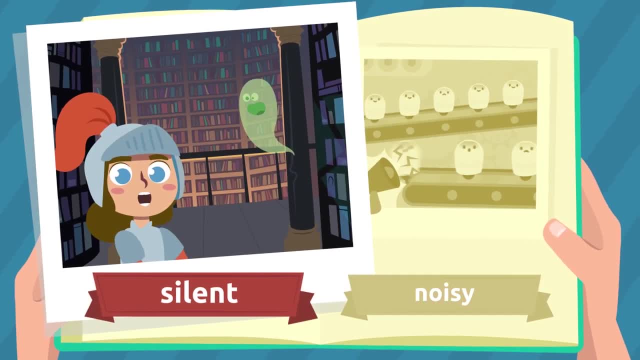 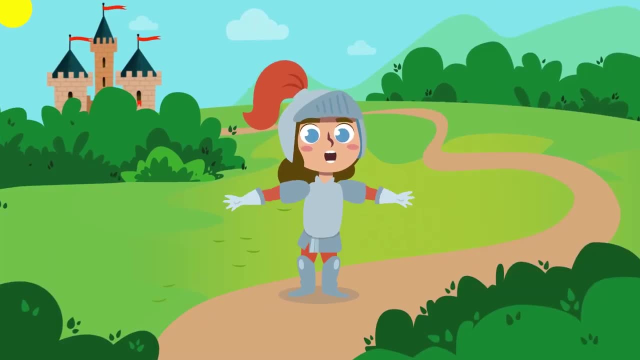 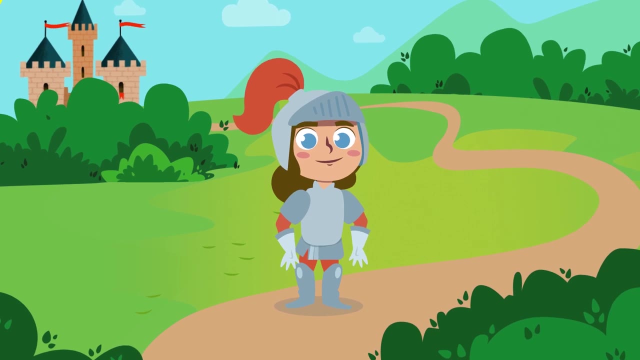 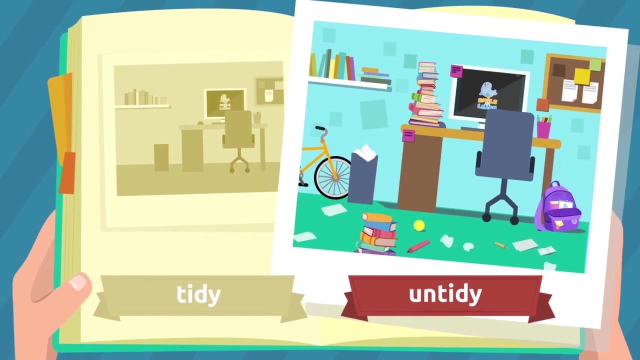 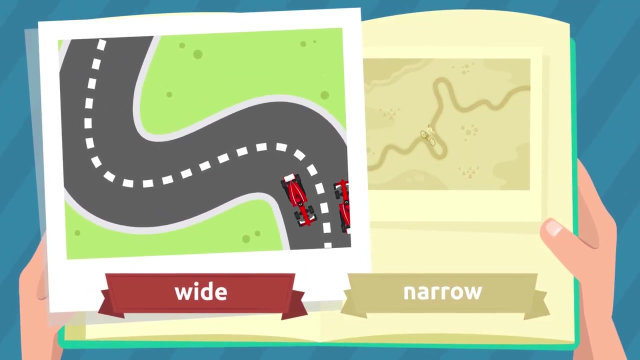 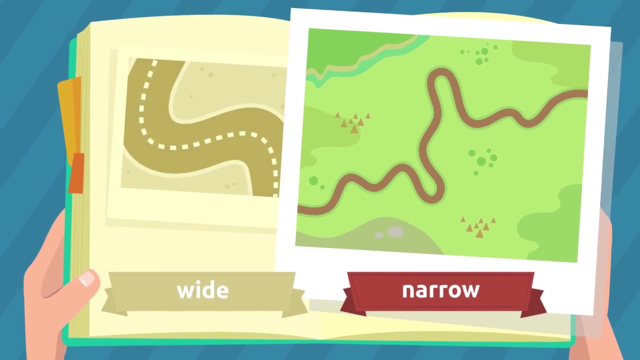 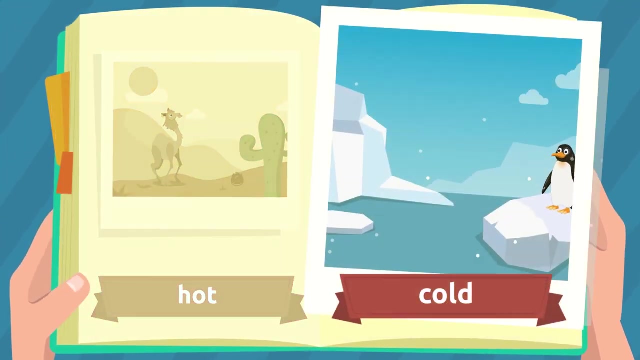 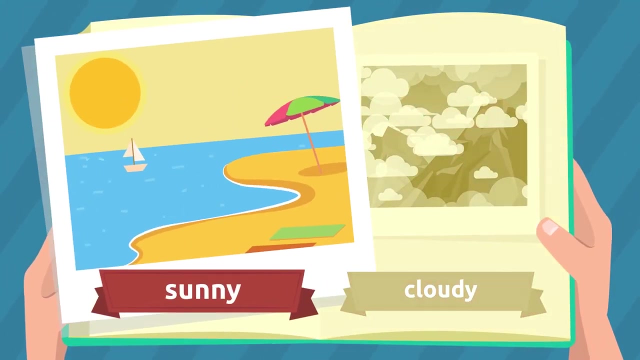 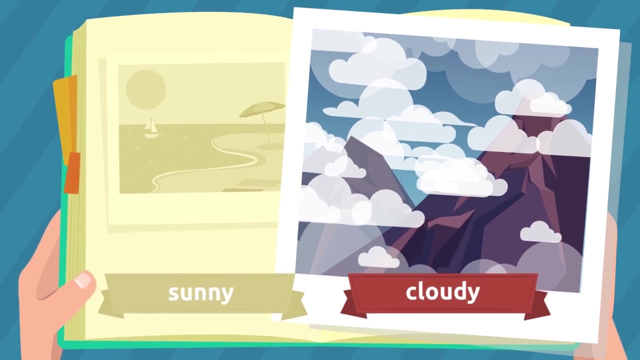 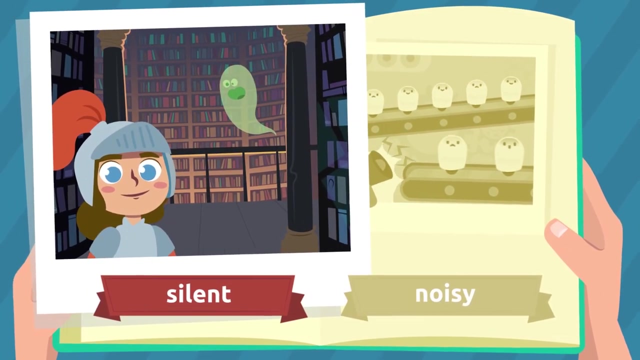 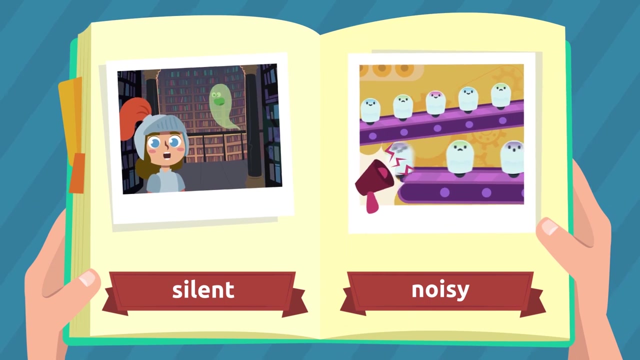 Silent Noisy. We've learned a lot of adjectives about these curious places. Let's review them. Tidy, Untidy, Untidy, Wide Narrow, Hot, Cold, Sunny, Cloudy, Silent Noisy, Nice work. 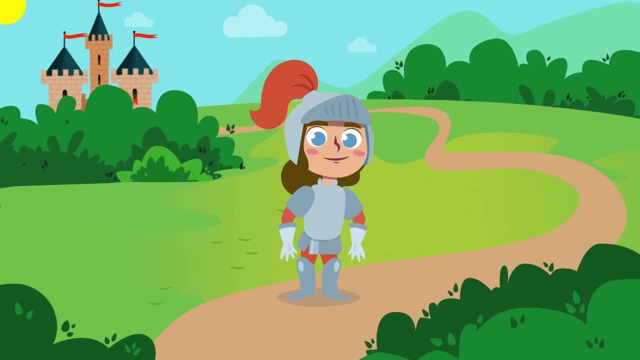 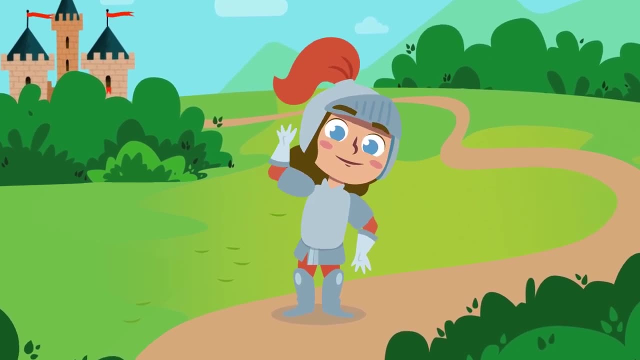 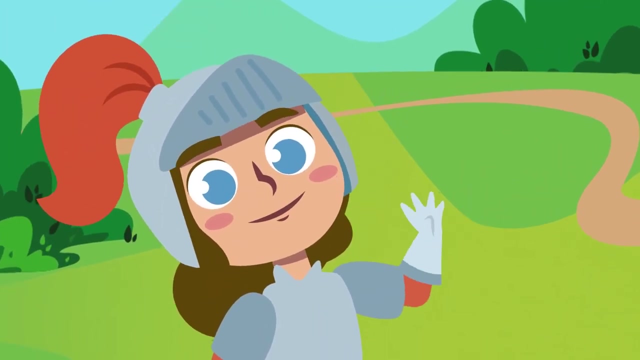 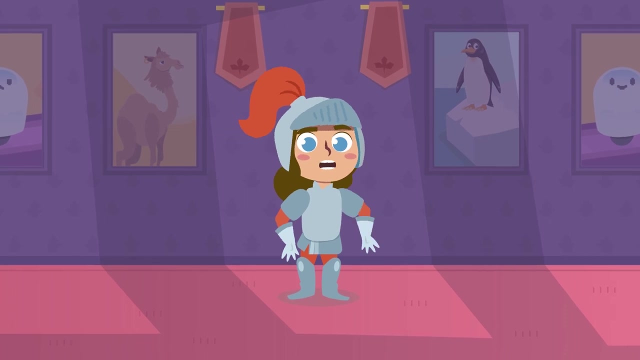 Adjectives are super fun. In this video we've learned a lot about them with some places. In the next episode we will learn more, But this time with objects. Don't miss out Greetings, word, lover friends. Today we will continue learning more adjectives. 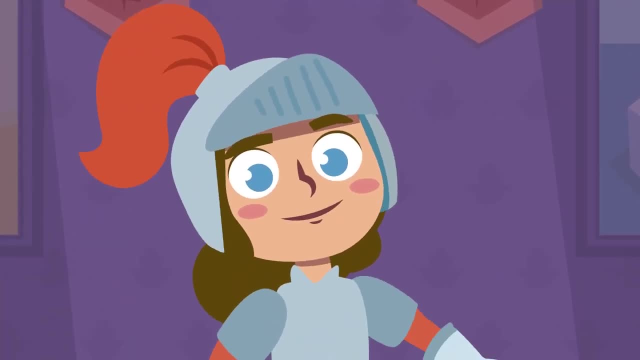 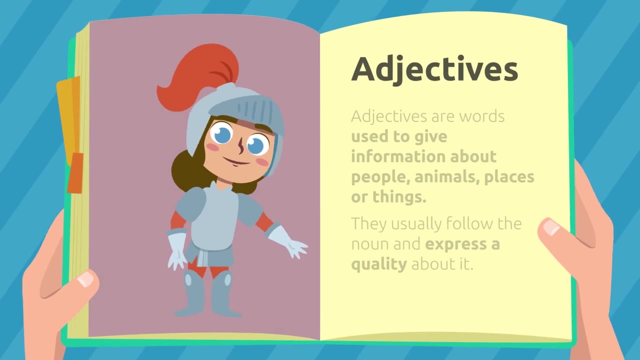 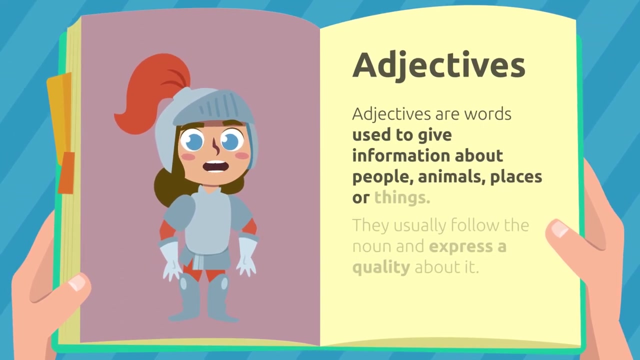 What do you say? Do you remember what adjectives are? Don't worry, I'll help you. Adjectives are words used to give information about people, animals, places or things. They usually follow the noun and express a quality about it. 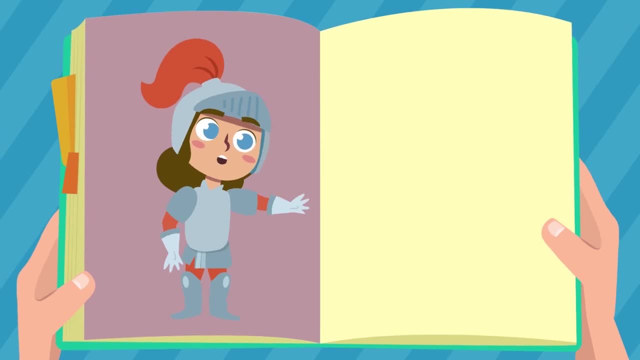 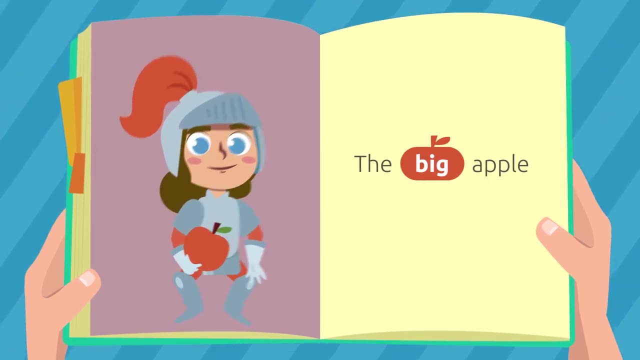 For example, in the sentence the big apple. Big would be the adjective because it tells us what the apple is like. In this video, we're going to learn some adjectives that describe qualities about different objects. Adjectives are words used to give information about people, animals, places or things. 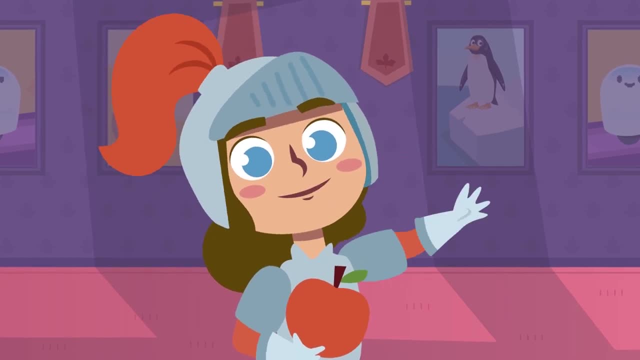 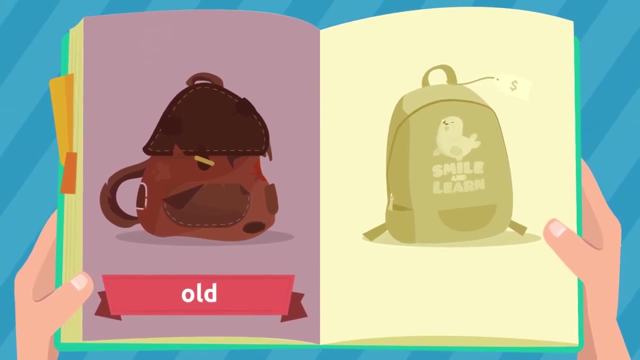 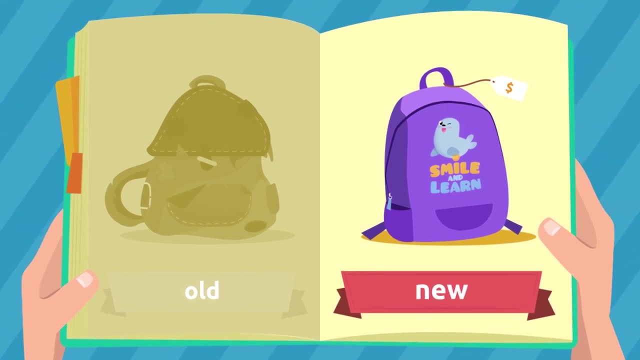 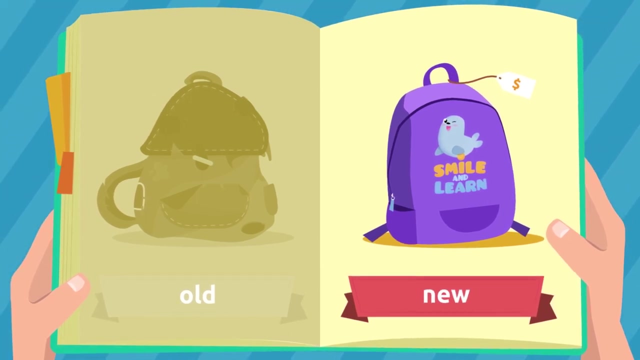 They usually follow the noun and express a quality about different objects. Let's begin. This backpack is old, Old, Repeat after me Old, But this backpack is new, New, Repeat after me New, But this backpack is old, New. 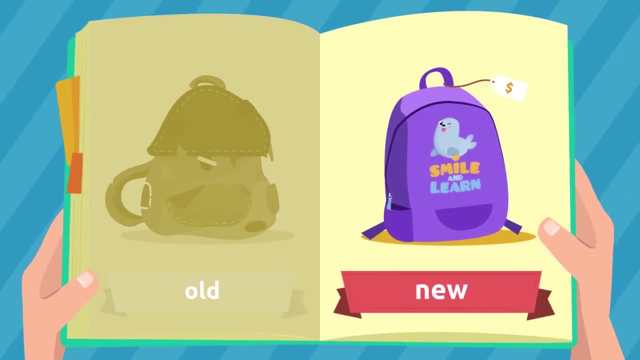 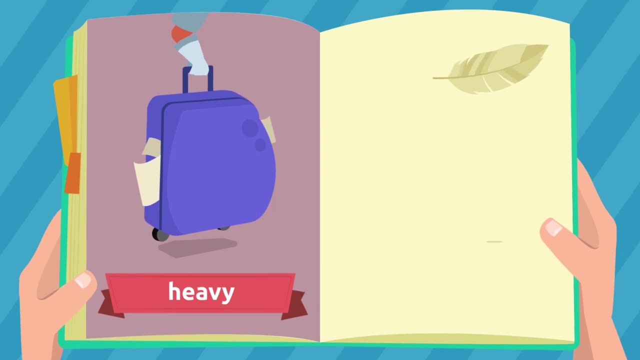 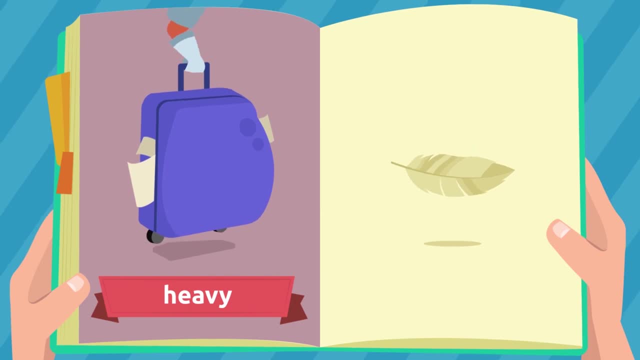 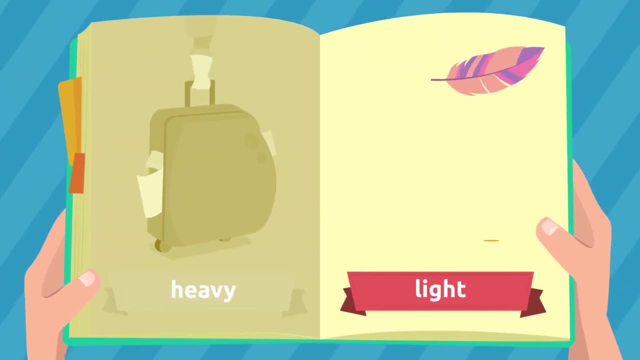 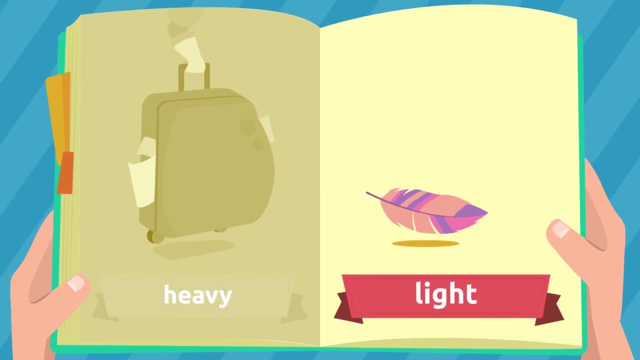 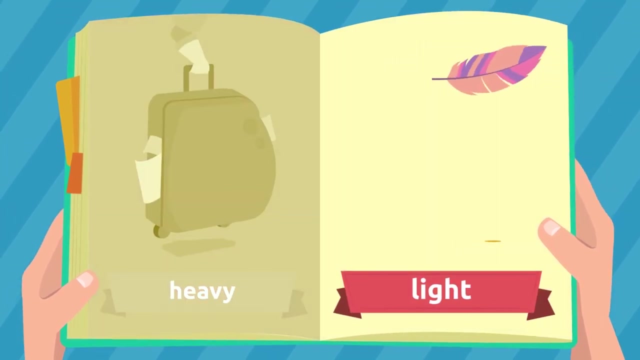 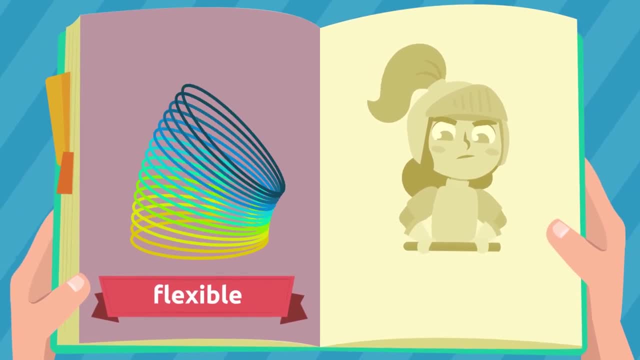 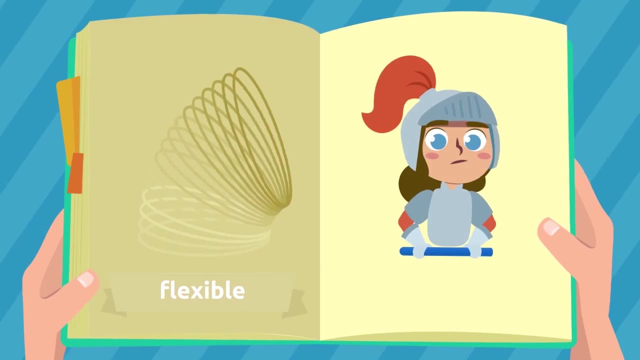 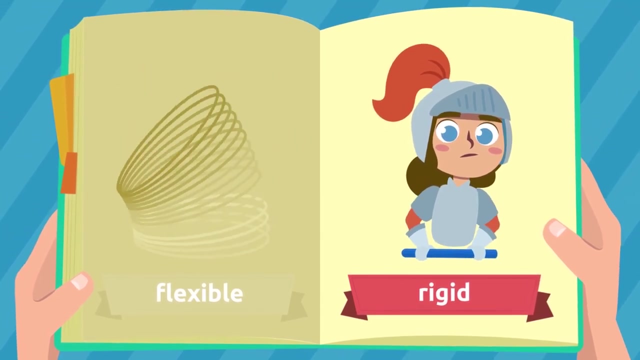 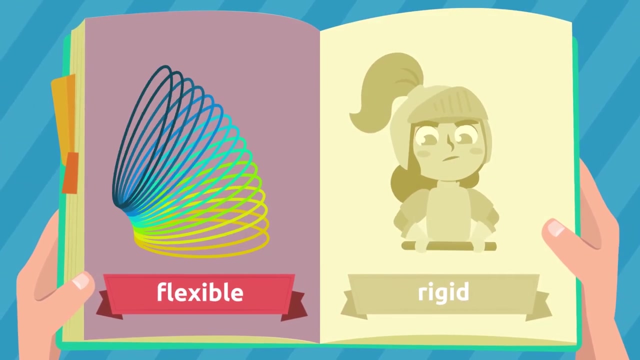 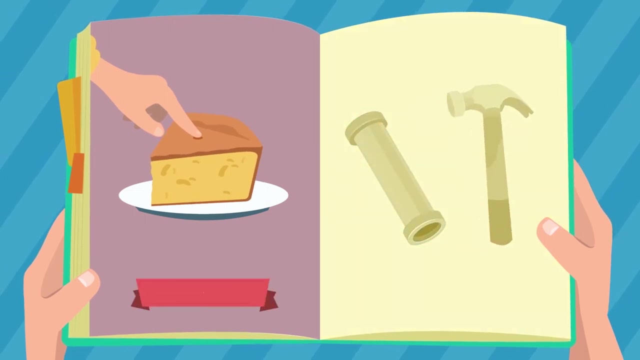 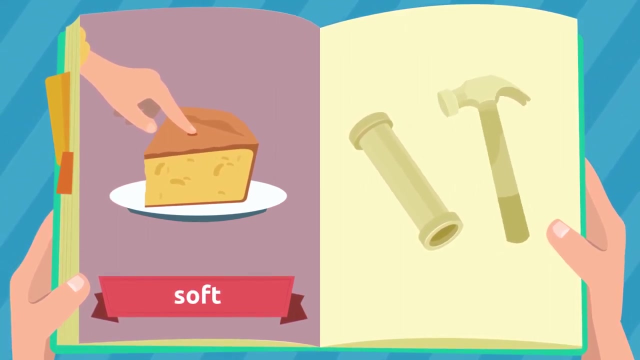 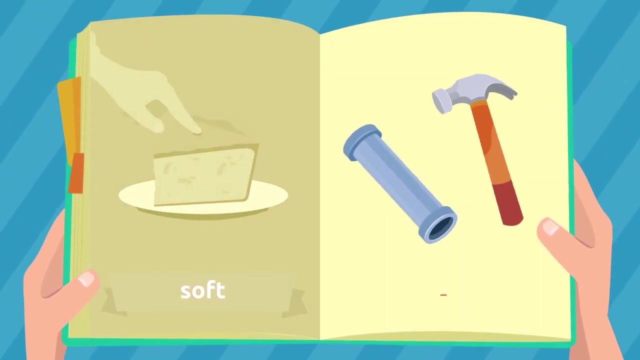 Flexible- Repeat after me Flexible, Flexible. But this steel bar is rigid, Rigid- Repeat after me- Rigid, Flexible, Rigid. This cake is soft, Soft, Repeat after me Soft. And this hammer is hard. 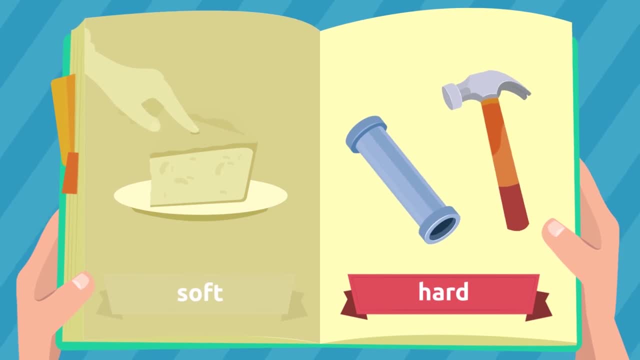 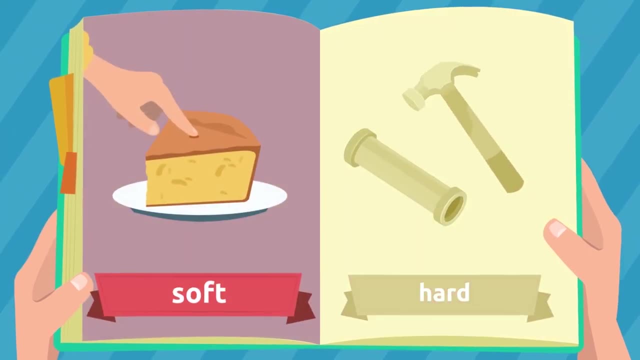 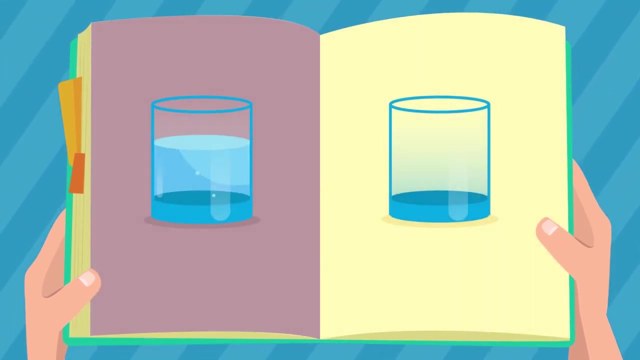 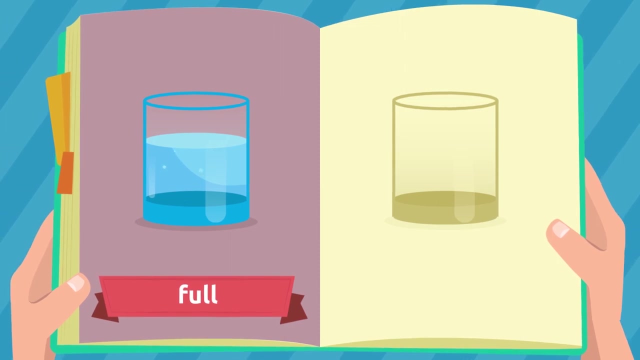 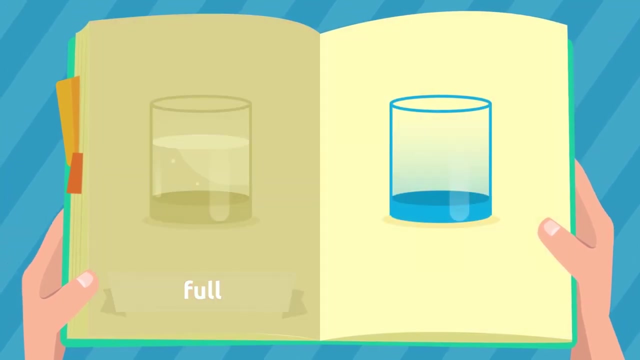 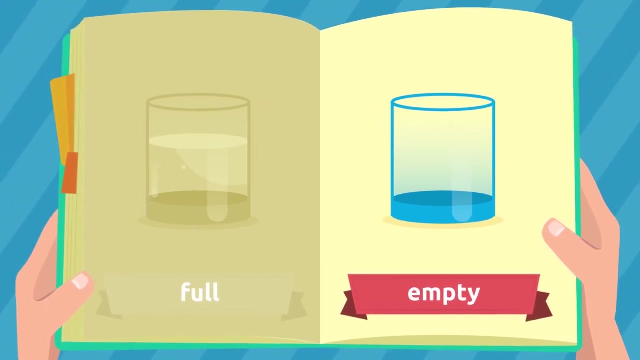 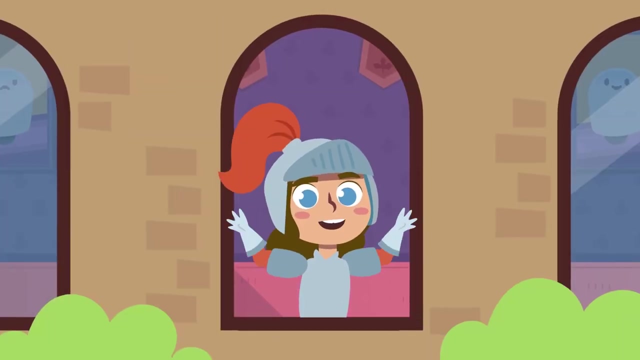 Hard- Repeat after me Hard, Soft, Hard, Hard. This glass Is full- Full- Repeat after me Full. But this glass is empty- Empty- Repeat after me Empty, Full, Empty. We've learned a lot of fun adjectives about these objects. 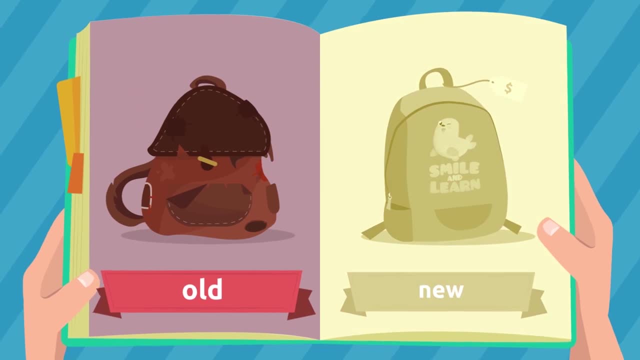 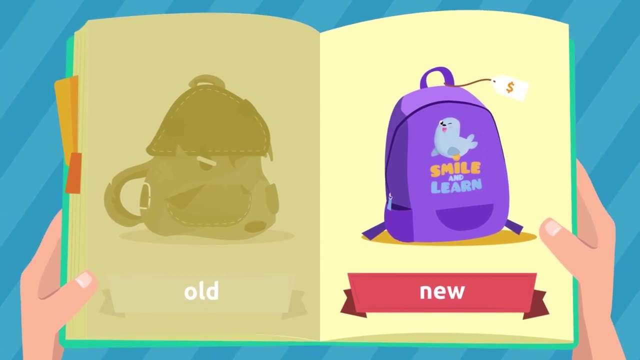 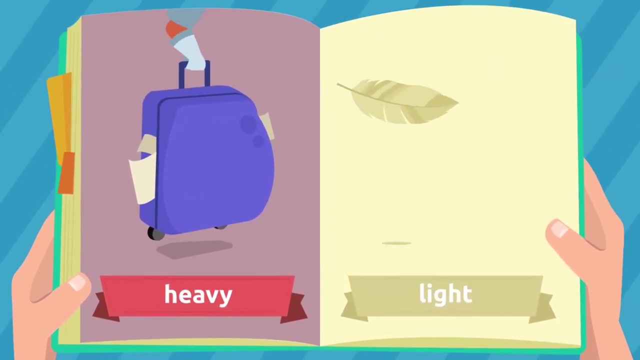 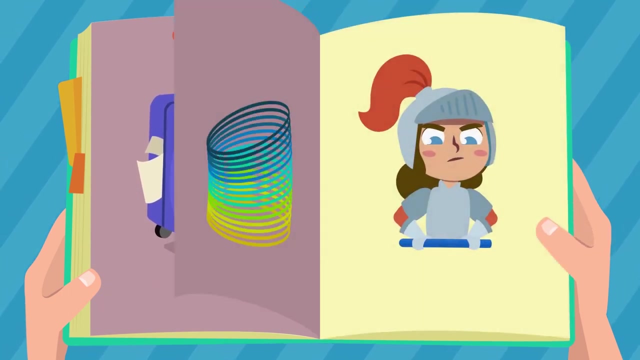 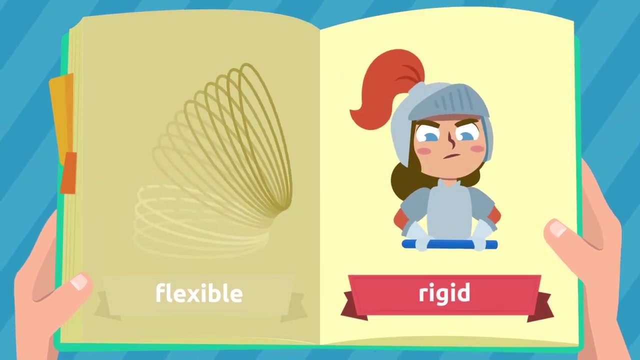 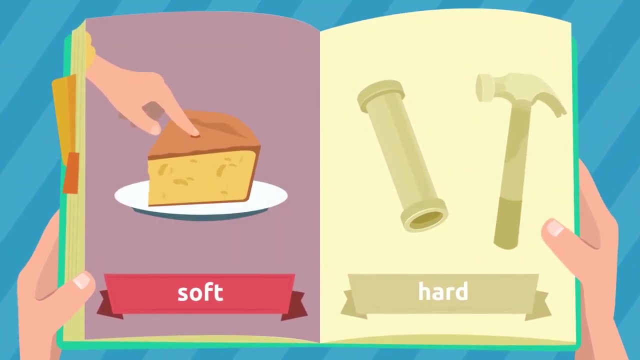 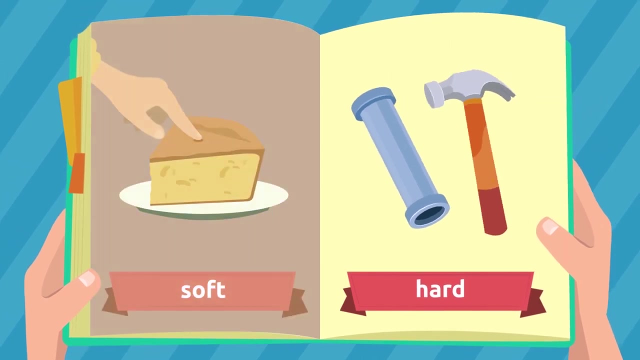 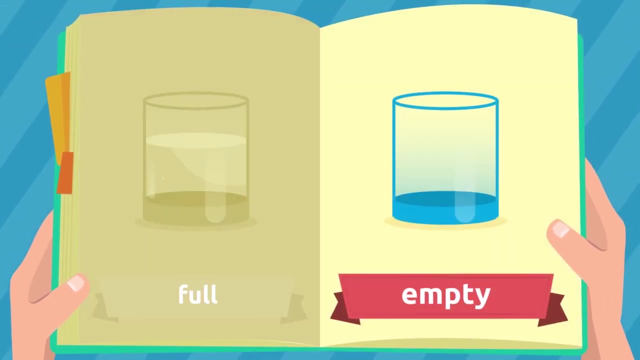 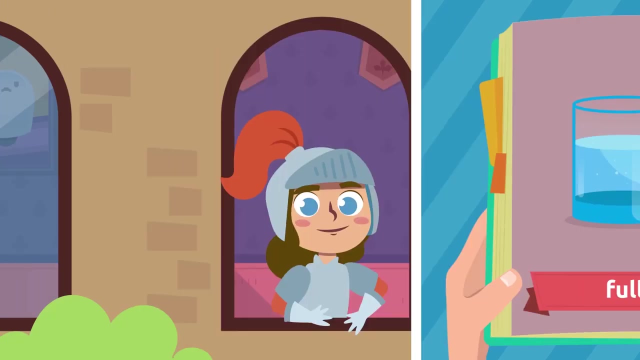 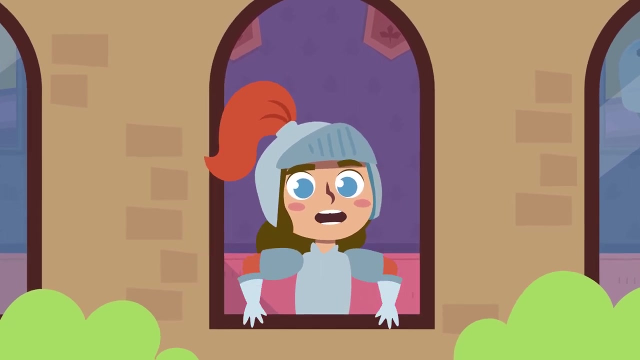 Let's review them: Old, New, Heavy, Light, Flexible, Rigid, Soft, Hard, Soft, Full, Empty, Great job- Adjectives are super fun. In this video we've learned a lot about them by talking about some objects. In the next episode we'll learn more. 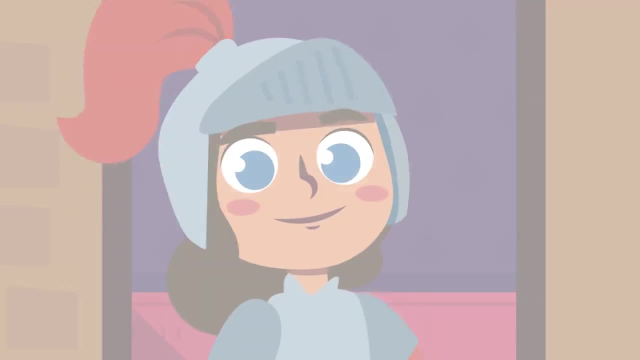 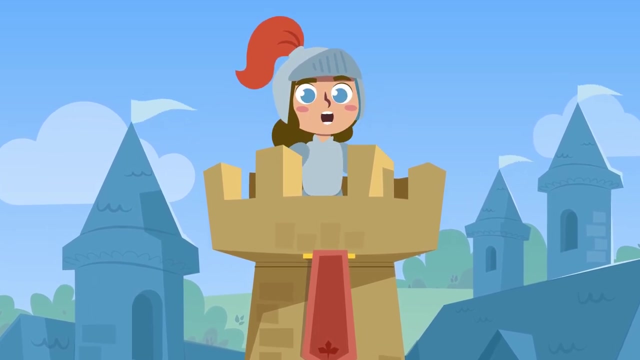 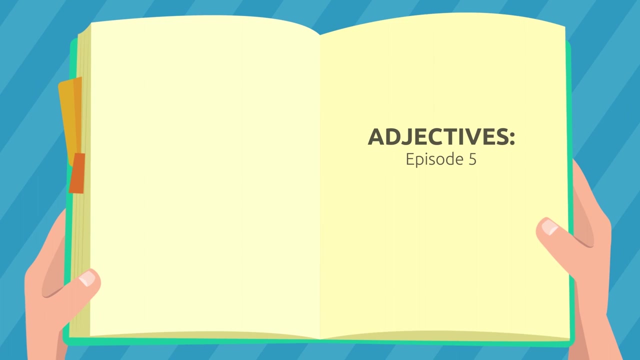 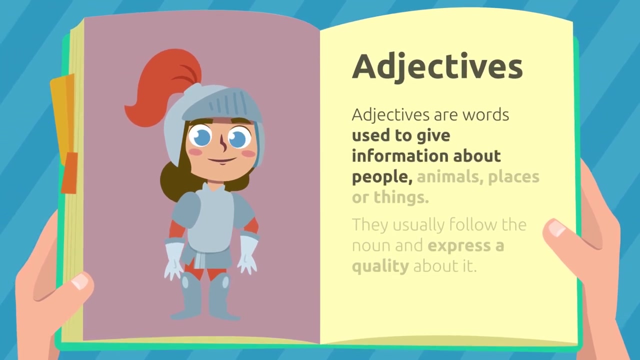 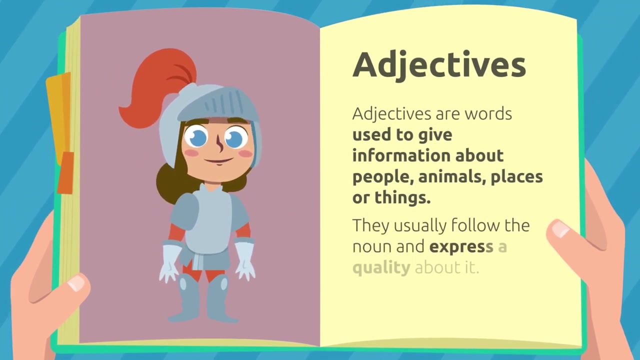 So don't miss it. Adjectives are words used to give information about people, animals, places or things. They usually follow the noun and express a quality of the word. They usually follow the noun and express a quality of the word. Adjectives are words used to give information about people, animals, places or things. 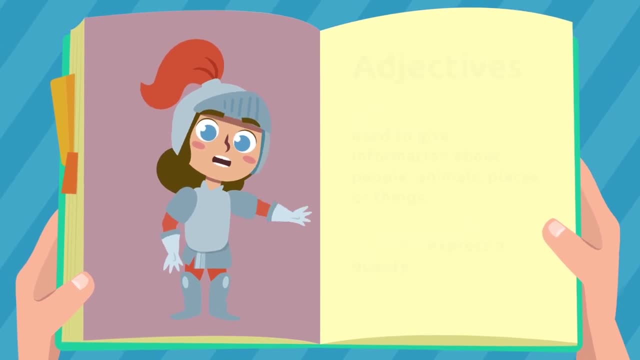 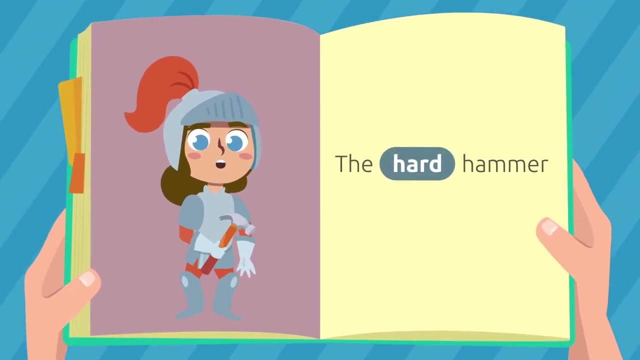 They usually follow the noun and express a quality of the word. They usually follow the noun and express a quality of the word. For example, in the sentence, Hard would be the adjective because it tells us what the hammer is like In this last episode. 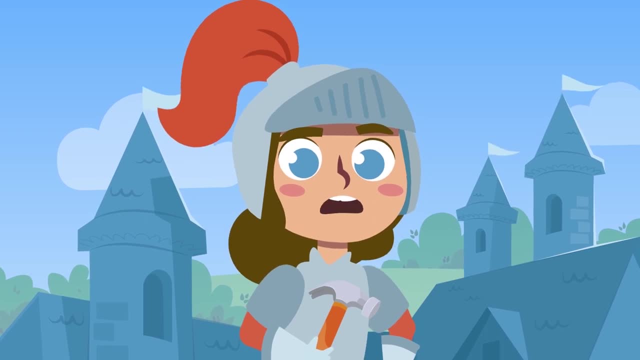 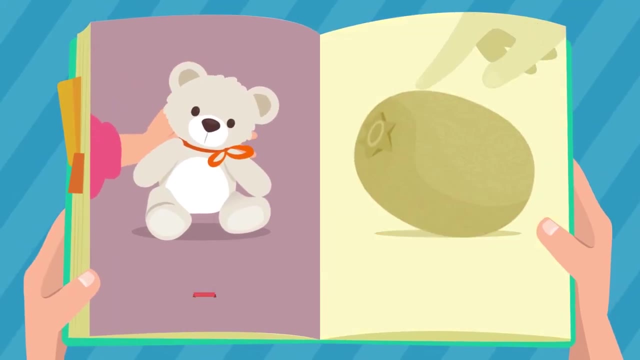 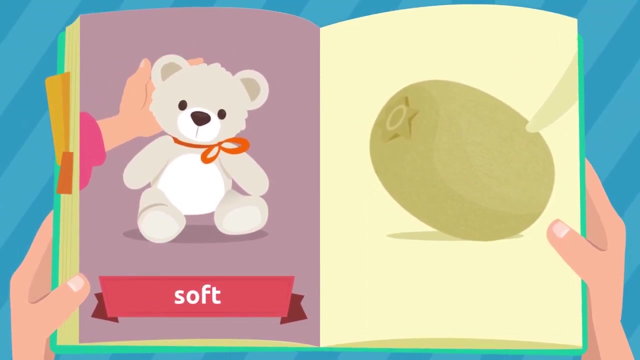 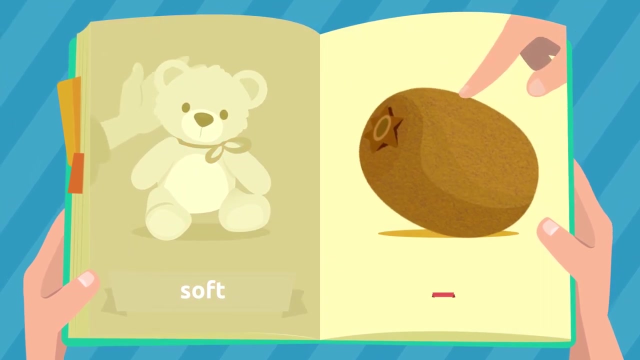 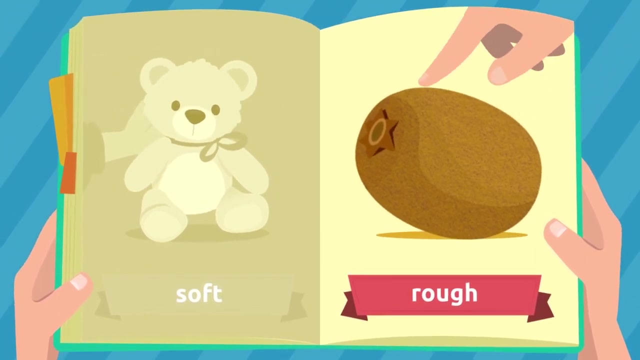 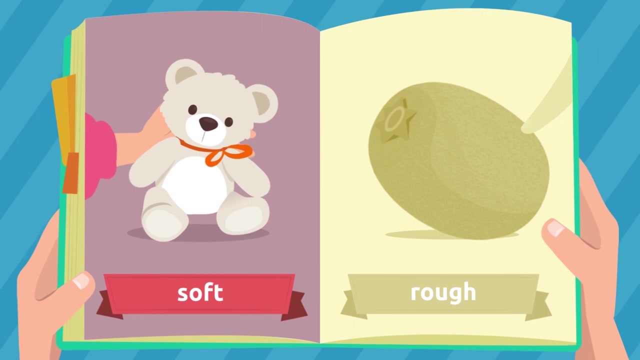 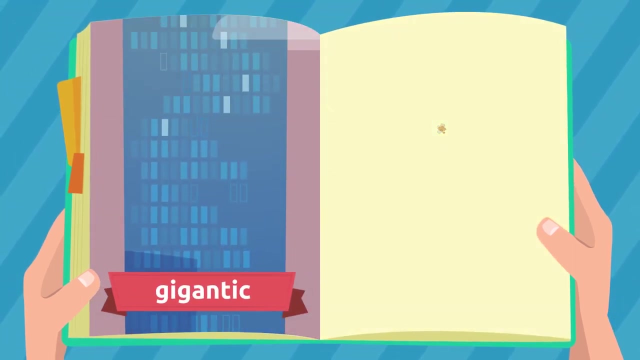 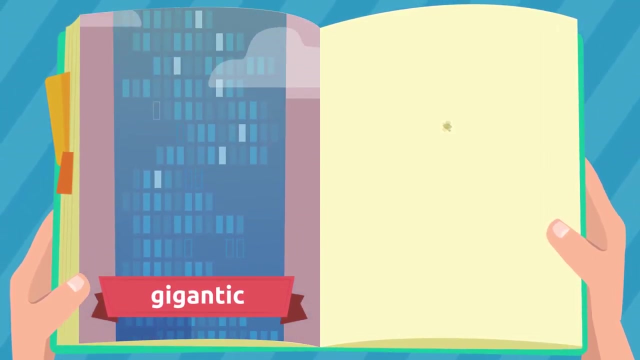 we're going to learn about some adjectives that we use to describe qualities about different objects, So let's get started. This stuffed animal is soft, Soft- repeat after me soft. and this Kiwi is rough, rough- repeat after me rough, soft, rough. this skyscraper is gigantic, gigantic- repeat after me gigantic. but 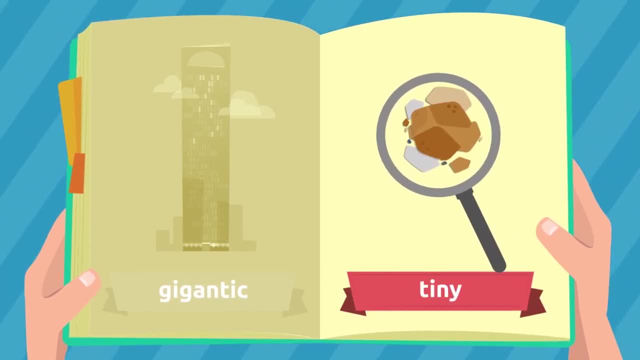 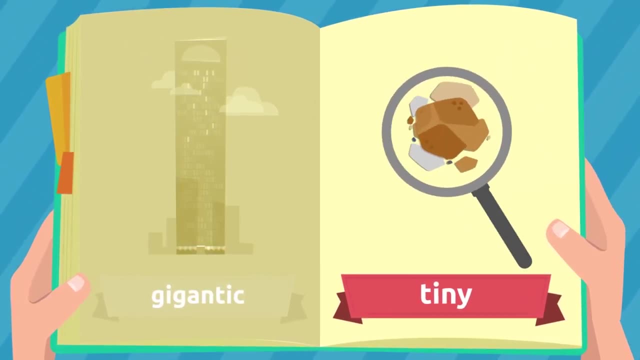 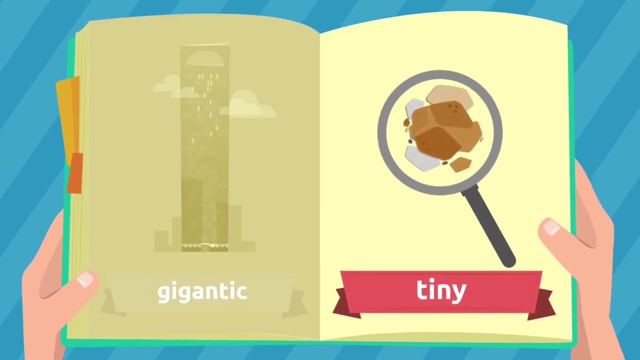 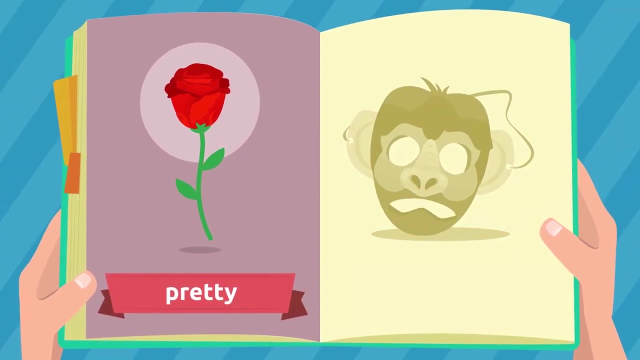 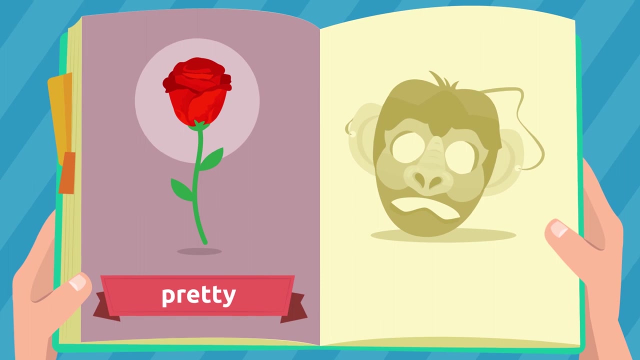 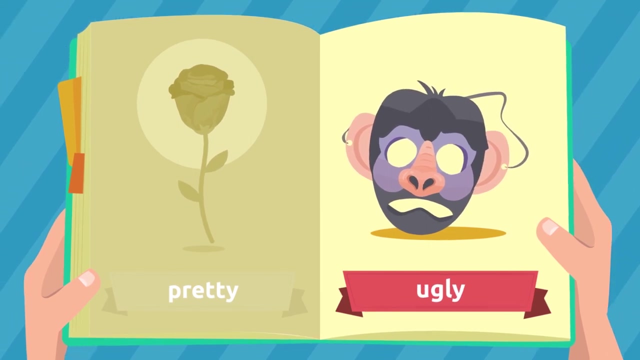 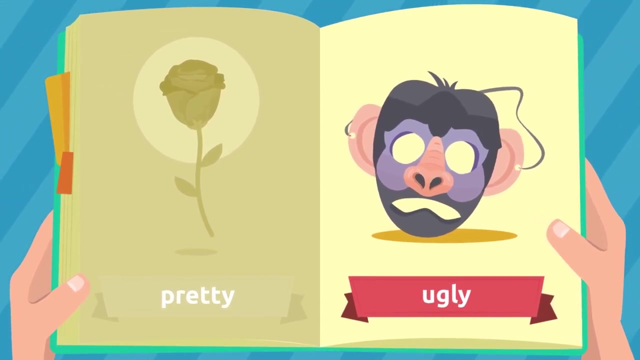 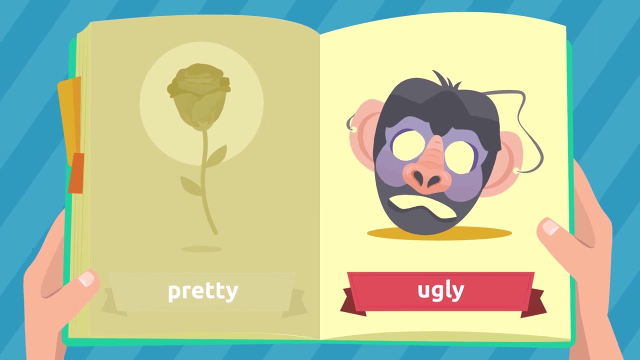 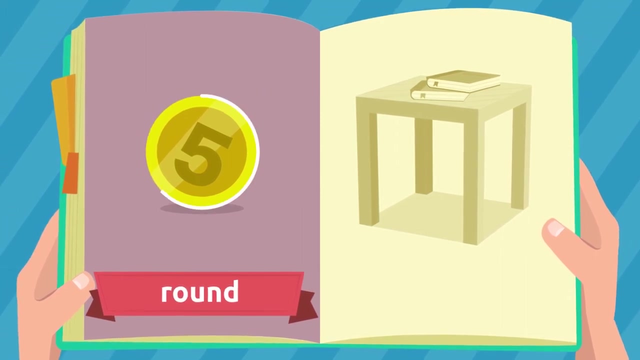 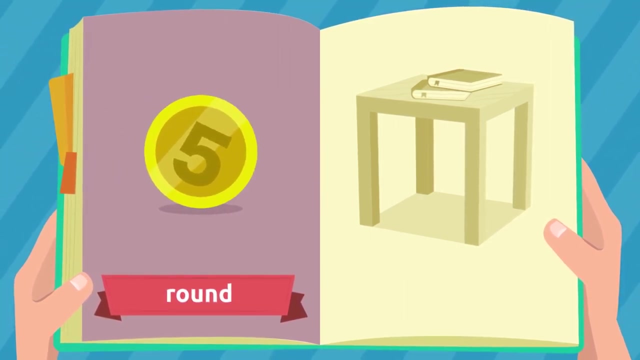 this grain of sand is tiny, tiny- repeat after me: tiny, gigantic tiny. this flower is pretty, pretty, repeat after me: pretty. but this mask is ugly, ugly- repeat after me: ugly, pretty, ugly. this coin is round, round. repeat after me: round and this coin is round, round. repeat after me: round and this. 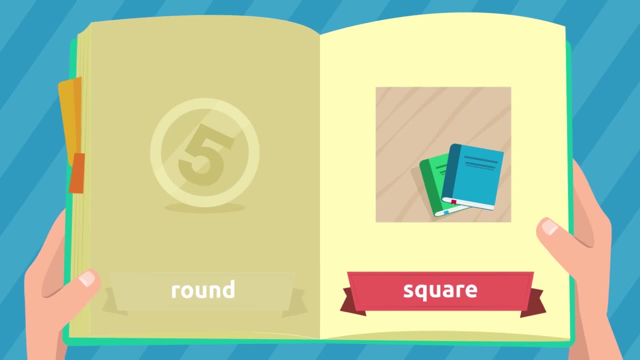 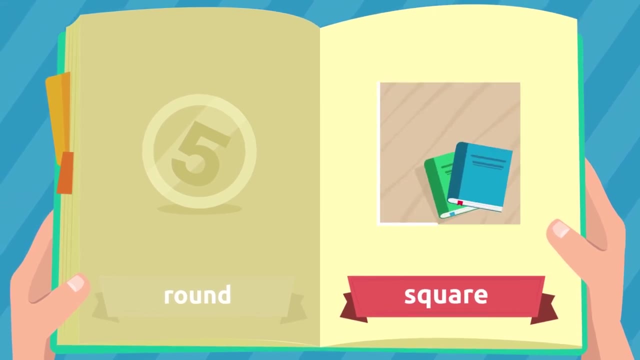 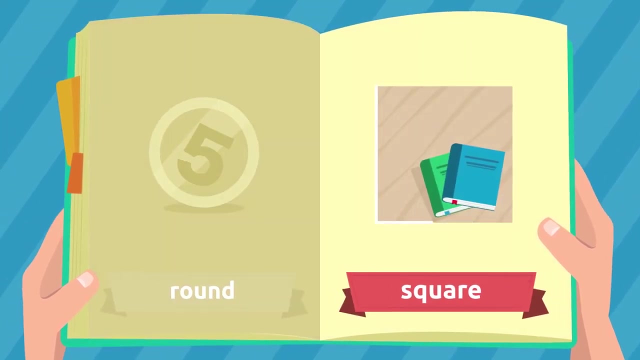 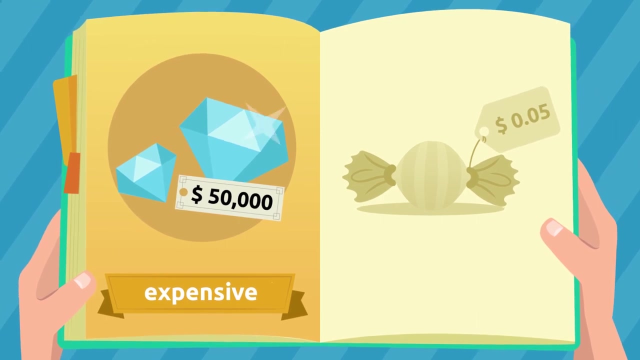